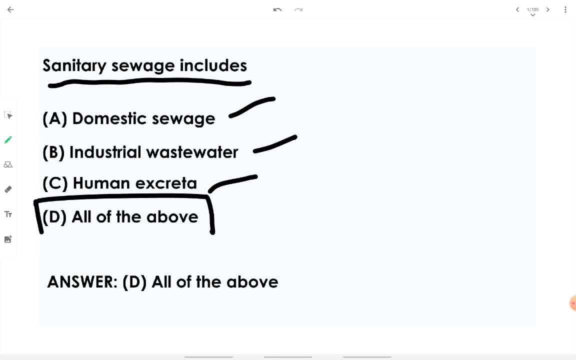 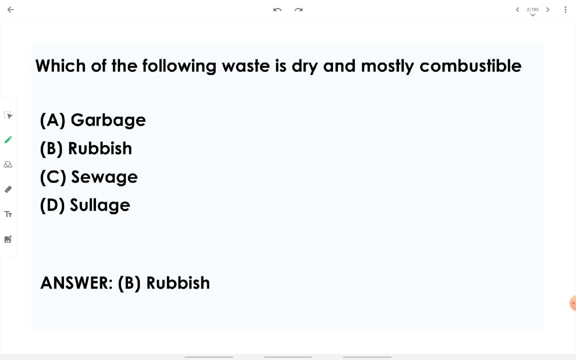 That's why sanitary sewage is comprising of all of the above. Therefore, option D is the correct answer. Let's go to question number next. Which of the following waste is dry and mostly combustible? See, rubbish contains least moisture content and it's mostly combustible because of the low moisture content in it. 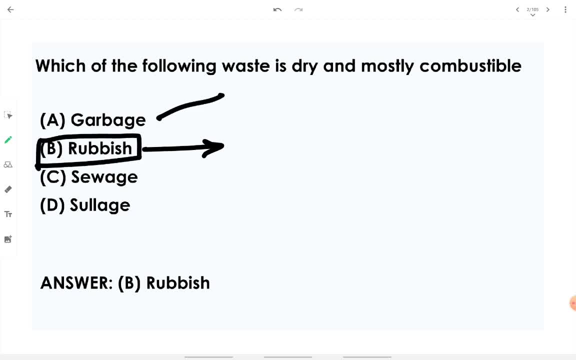 OK, that's why the rubbish is the answer here. Garbage consists of organic, inorganic waste, and organic waste mostly consists of vegetables and other waste products that are having more moisture content. Sewage: obviously it is. Westwater. Sallage, obviously kitchen waste. 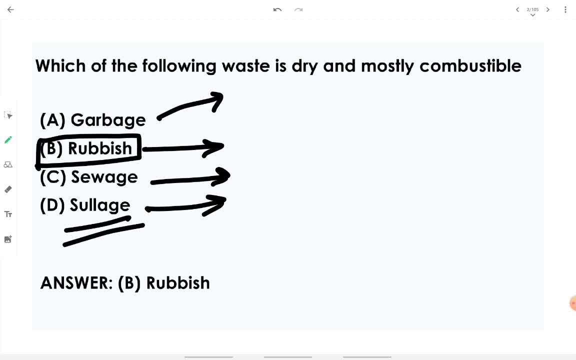 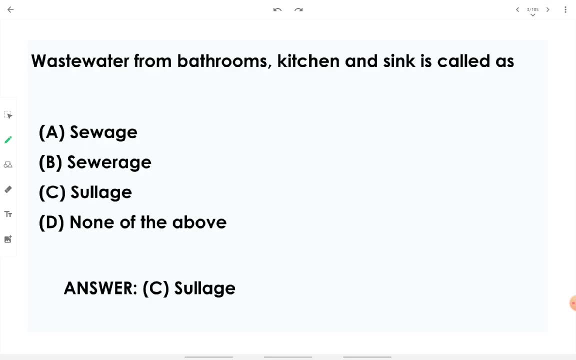 You know, since it is Westwater, moisture content is too high in sallage, sewage and garbage. That's why they are not combustible. Rubbish becomes the correct answer here. OK, Then waste water from bathrooms, kitchen and sink. 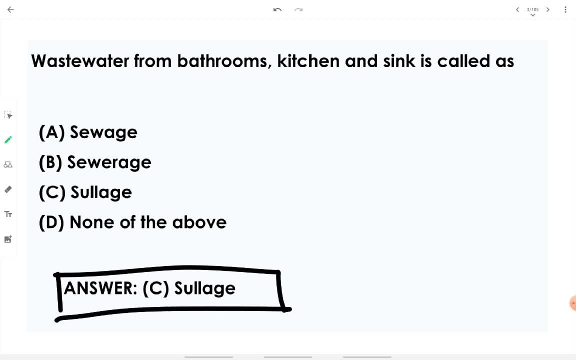 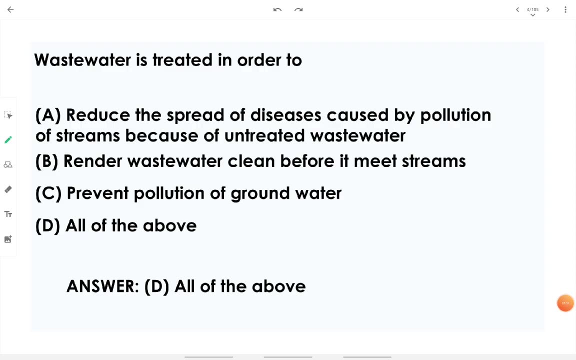 Collectively it is called as sallage. OK, Remember the word sallage. It is the waste water from bath- OK. Then kitchen and sink- OK, It is called as sallage. So waste water is treated in order to reduce the spread of disease caused by pollution of stream because of untreated waste water. 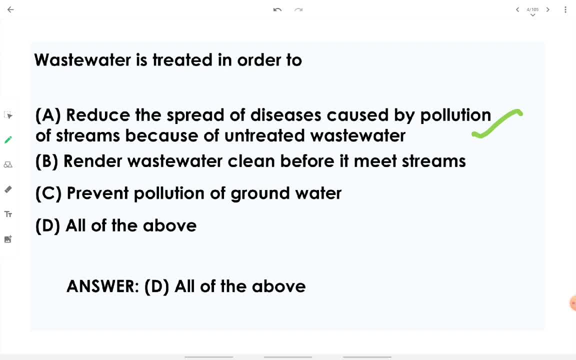 Yes, if untreated waste water meets the river stream, then it will not only cause pollution but it will spread diseases. OK, then it will render the waste water clean before it meets the stream. Yes, waste water should be first treated, then should be released into the stream- natural stream. 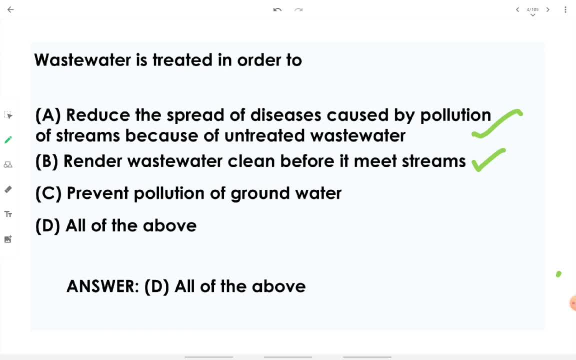 So that they will undergo dilution and self-purification, thereby causing total cleansing of water. OK, Therefore, the water- waste water- should be cleaned. It should be rendered clean before it is meeting natural river stream or any stream of water. 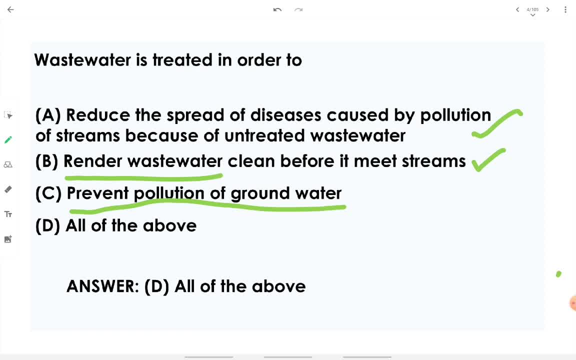 It prevents pollution of groundwater. OK, If waste water is left untreated, what will happen? It will reach the groundwater source and it is going to cause pollution of the groundwater, And consumption of such groundwater is going to lead to some disease or any pandemic. 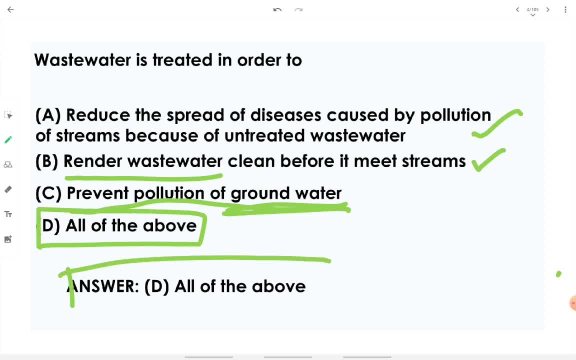 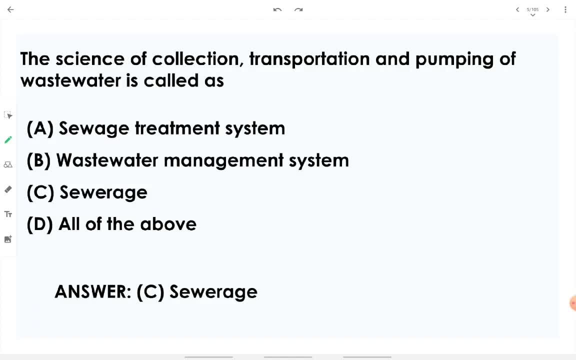 That's why all of the above becomes the correct answer here. OK, let's go to question number next. The science of collection, transportation and pumping of waste water is called as OK. sewerage is the science of collecting the waste water, transporting the waste water through sewers. 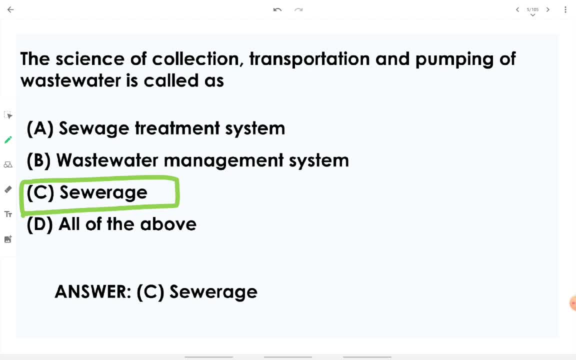 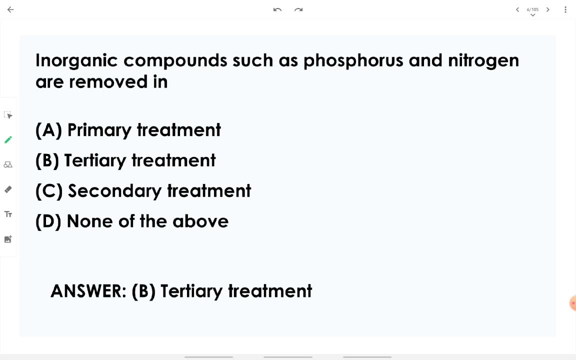 OK. and pumping the waste water toward the exit point: OK. The whole system of collecting, transporting and pumping is called as sewerage. Then inorganic compounds such as phosphorus and nitrogen are removed in tertiary treatment- OK, The most advanced treatment stage is the tertiary treatment. 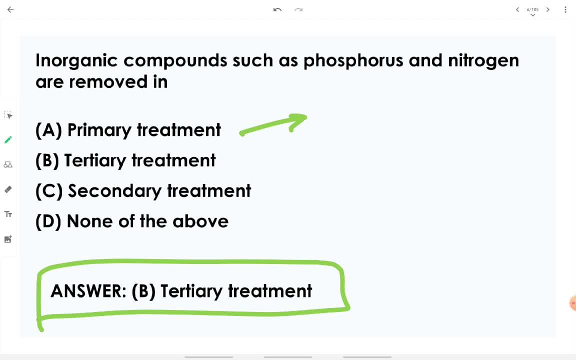 In primary treatment. what we are removing? We are removing floating debris, then grit is there, then axial there. Obviously, whatever the floating debris which are coarse in size and whatever the heavy material having more specific gravity are removed in primary treatment. 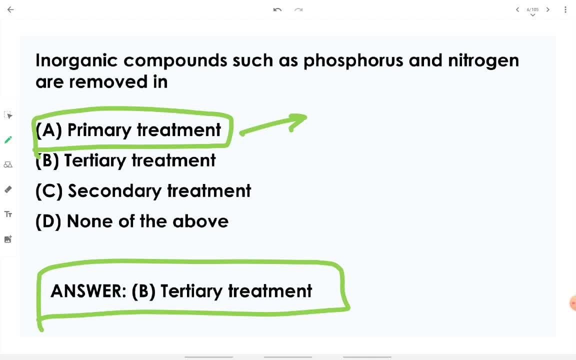 Such as detritus tank. is there, then, screening chamber? is there? OK, then shredding of the content in waste water is there. It is done in primary treatment, Then in secondary treatment. what we are going for? We go for biological treatment of waste water. 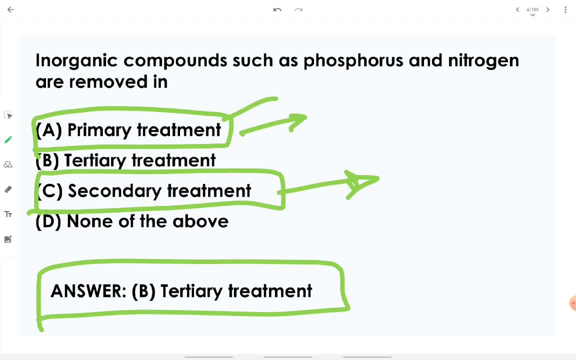 It is done in secondary treatment, Just like activated sludge process. is there? trickling filter is there? then the rotating biological contactors are there. they are part of secondary treatment. In tertiary treatment, the most advanced treatment available is in which we can separate the minerals. 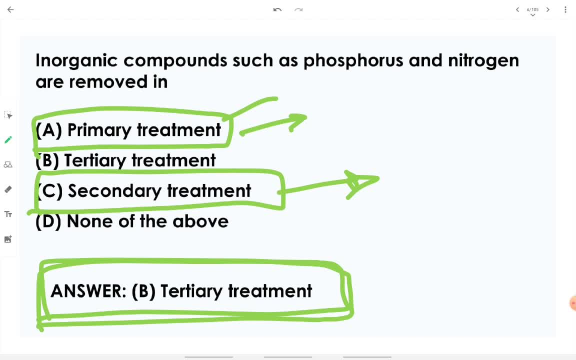 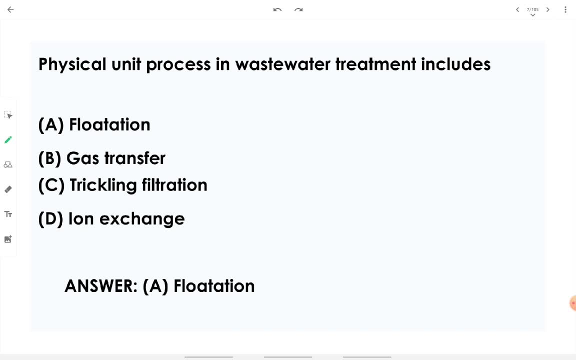 which are present in waste water. OK, Therefore inorganic compounds such as phosphorus and nitrogen are removed in tertiary treatment. Then physical unit process in waste water treatment includes- Yes, it does include- flotation process. OK, Gas transfer is a molecular level, chemical level kind of process. 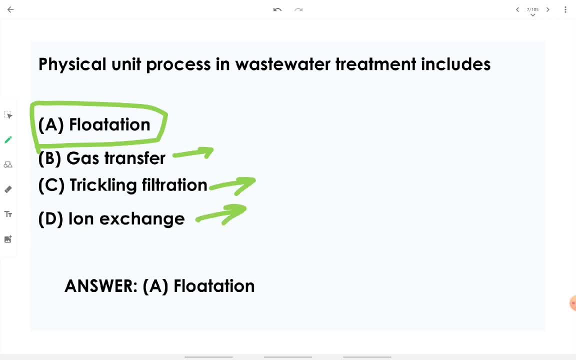 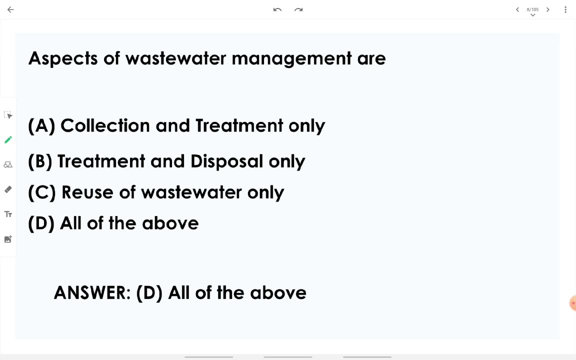 Trickling filter: It is a biological process. Ion exchange: again it is a chemical process. Therefore, the only physical process we have been provided in the option is flotation. OK, let's go. Question number next Aspect of waste water management are collection, treatment, disposal, reuse and recycle. 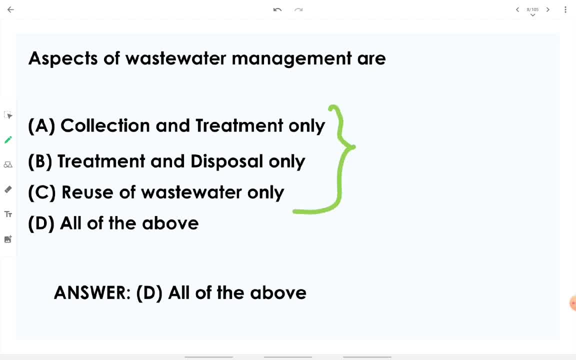 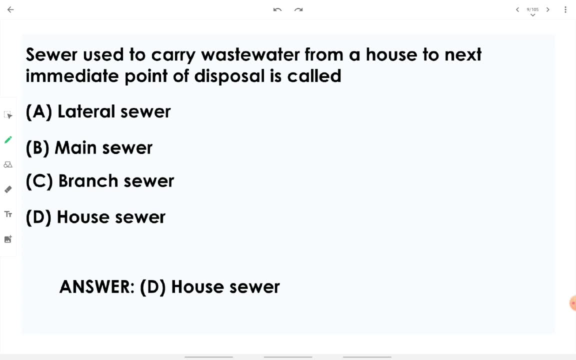 And all the three options here are saying: collection, treatment, disposal, reuse, recycle. OK, therefore, the most correct answer here becomes all of the above. OK, let's go to question number next. Sewer used to carry waste water from a house to next immediate point of disposal is called as house sewer. 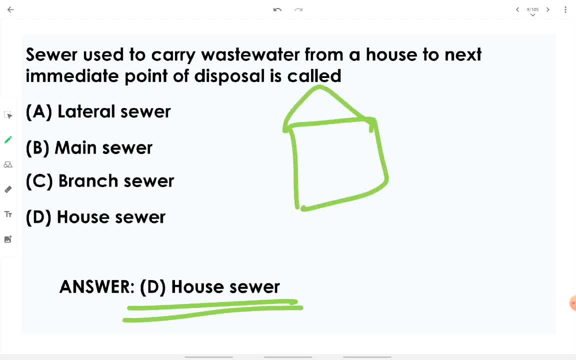 OK, for example, a house is there, Then whatever the waste water that is coming out of the sewer is house sewer, And after the house sewer, the multiple house sewers are connected to the lateral one. OK, we will see the same point in next questions. 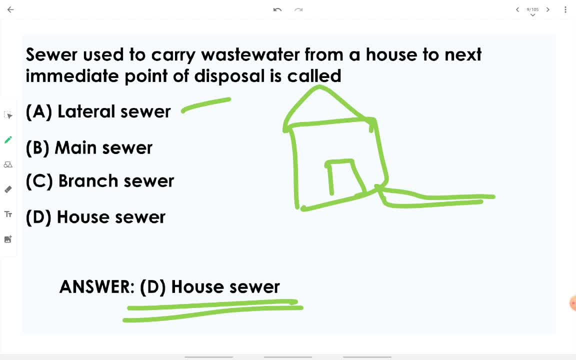 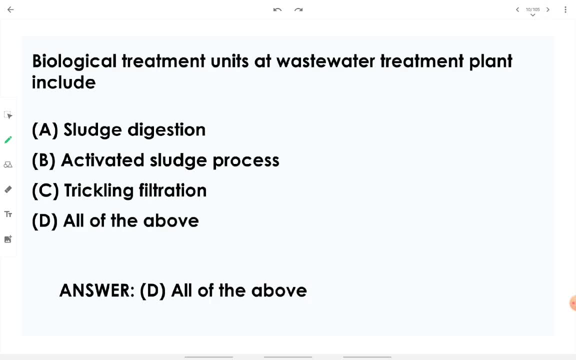 OK, remember, sewer, which is carrying waste water from a house to next immediate point of disposal, is called as house sewer. Then biological treatment units at a waste water treatment plant include- Yes, they do include- solid digestion, which is the end process, activated sludge process, which is the biological process, trickling filtration. 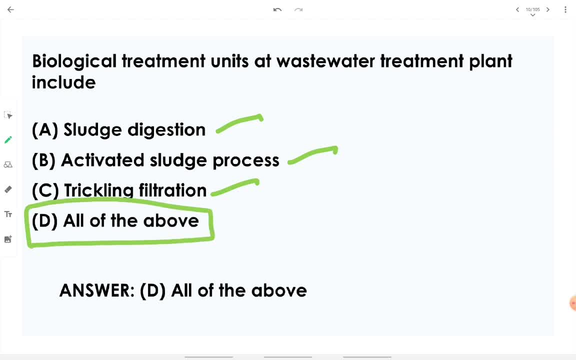 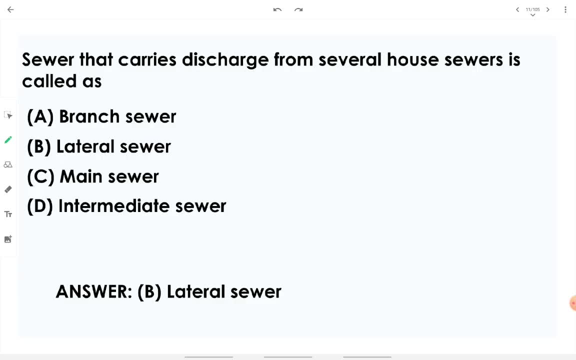 Yes, biological process. Therefore, all of the above mentioned processes or mentioned treatment units are present in waste water treatment plant. Then sewer that carries discharge from several house sewer is collected at. OK, is collected at where? at lateral sewer. OK, whatever the sewage is getting collected from house sewer is then disposed of to lateral sewer. 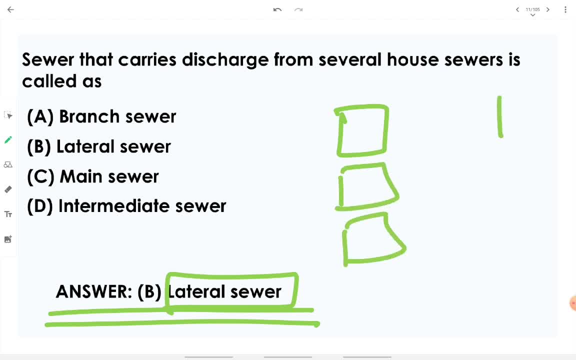 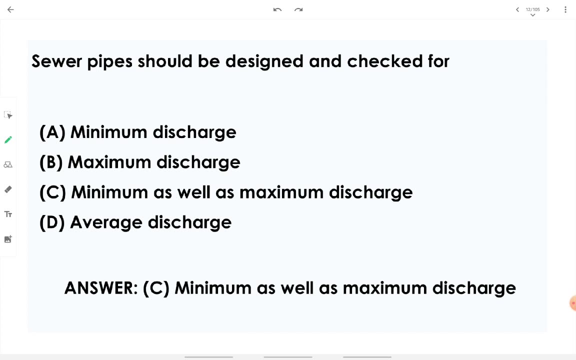 For example, number of houses are there and from those houses a lateral sewer will collect whatever the sewage it is given out by the house sewer. OK, this is the lateral sewer. OK, Then sewer pipe should be designed And check for minimum discharge and maximum discharge both. 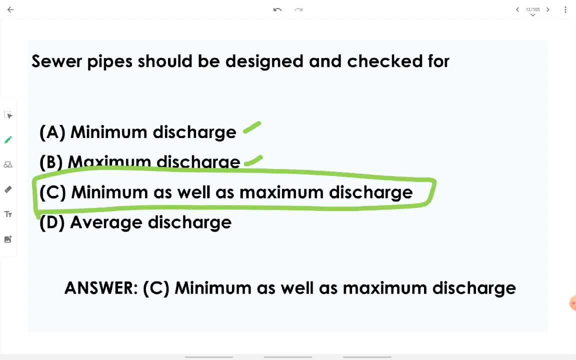 OK, therefore, option C is the good choice of correct answer. Minimum as well as maximum discharge- See. minimum discharge should be checked so that there should not be any clogging to happen or to take place inside the sewer which will restrict the regular. 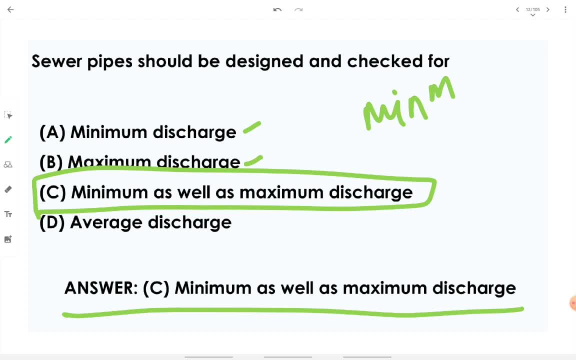 flow of wastewater through the sewer and maximum permissible discharge should be there. OK, maximum permissible discharge should be there so that they don't overflow, And the capacity of the overall area should be there. OK for minimum and maximum. both discharges should be checked. 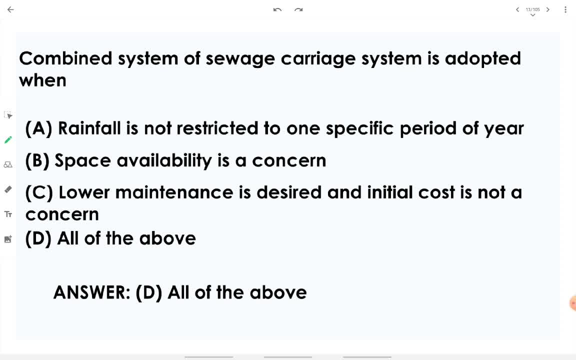 OK, Then combined system of sewage carrier system is adopted when rainfall is not restricted to one specific period of the year. Yes, we go with combined, not separated. when we are having rainfall throughout the year, OK, it is not restricted to several two to three months. 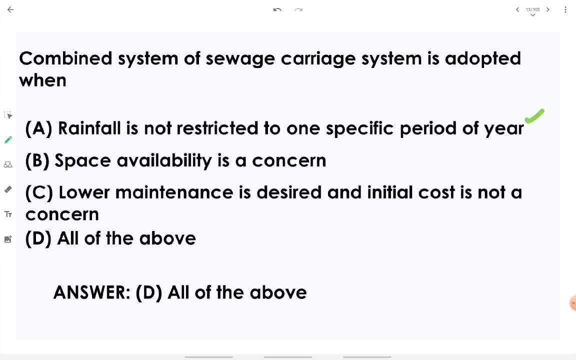 Therefore we will be requiring combined sewer system. OK, then space availability is constant. Yes, when we are providing two separate sewer, one for dry water flow and other for storm water flow, then space will be requiring. space requirement will be more. 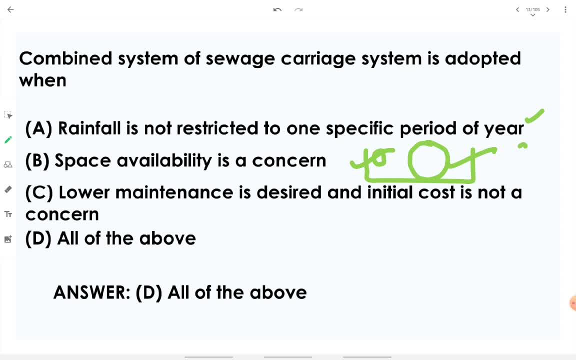 Therefore, instead of going for two separate sewer, we will go with a combined, a kind of large, one single kind of sewer over there. OK, then lower maintenance is desired. OK, when combined system maintenance is low but the initial cost is more in case, 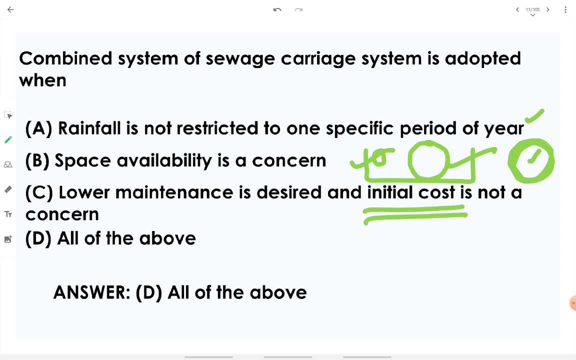 of combined system. initial cost, initial initial capital, starting capital is more in case of combined system. Therefore, it is adopted when option A, B, C, all are providing the conditions which are preferable for combined system. Therefore, answer D is the correct one. 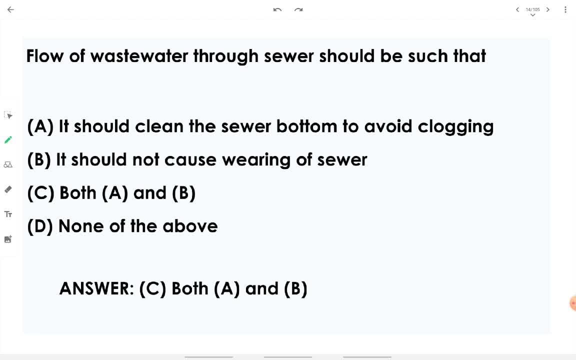 So flow of wastewater through sewer should be such that it should clean the sewer bottom to avoid clogging. Yes, Then it should not cause wearing of sewer. Yes, Minimum and maximum flow: OK. minimum and maximum velocity: OK, then the minimum velocity is the cleansing velocity. 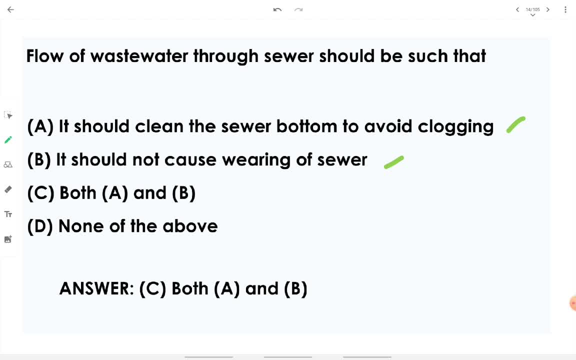 OK, self cleansing will take place only when the sewer is having the minimum Velocity, minimum restricted velocity over there. OK, and maximum permissible velocity that should be allowed in a sewer should be such that it will not cause wearing of the sewer. OK, wearing means scoring. action in scoring. 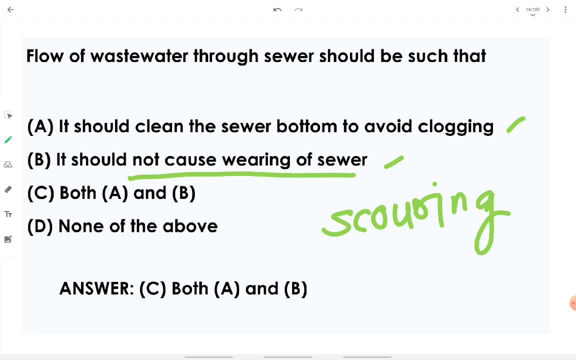 What will happen? The fast flowing wastewater will be taking off or will be disintegrating the surface of the sewer in which it is in contact with. OK, what will happen because of that? it will cause scoring or wearing or abrasive effect. It will cause abrasive. 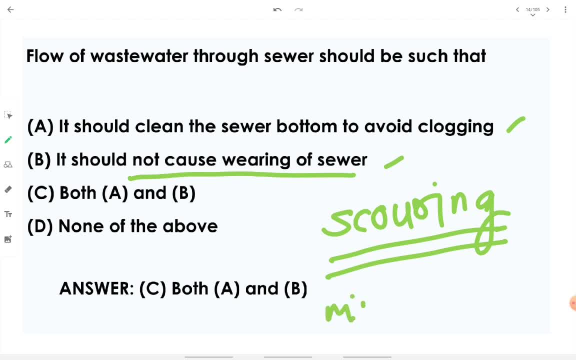 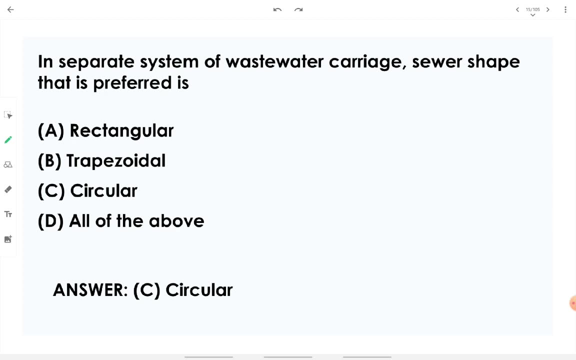 On the sewer. therefore, it should be check for minimum and maximum. Therefore, the minimum velocity is to have cleaning and maximum velocity should be such that it should not cause wearing. therefore, both A and B form the correct answer, Then, in separate system of wastewater. 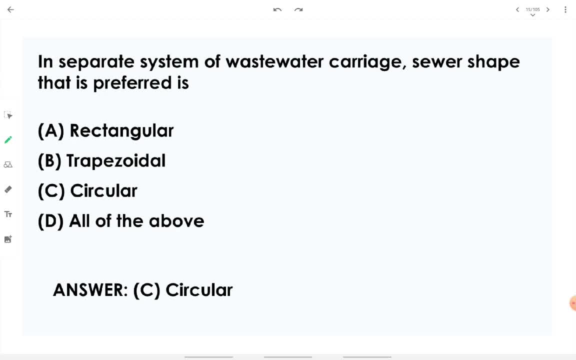 carriage. sewer shape which is preferred is circular: OK, in separate system. means for dry weather flow and for stormwater flow. the separate systems are such that their shape mostly preferential, which is circular, OK, circular sewers are preferred in separate system of wastewater carriage. 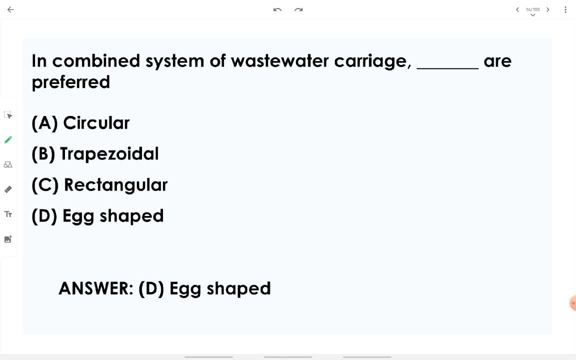 In combined system of wastewater carriage, egg shaped sewers are preferred. OK, in combined system, egg shaped sewers are preferred. They are just like this. Therefore, this makes the crown portion and this is the bulging portion in the egg shaped sewers. 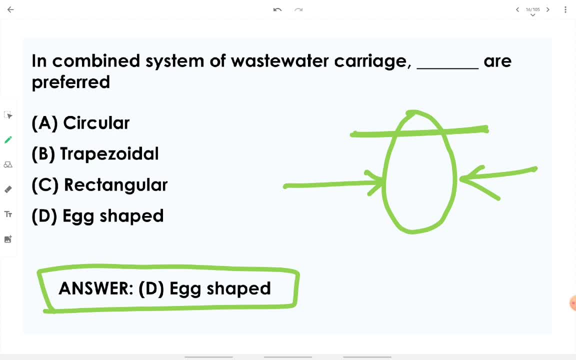 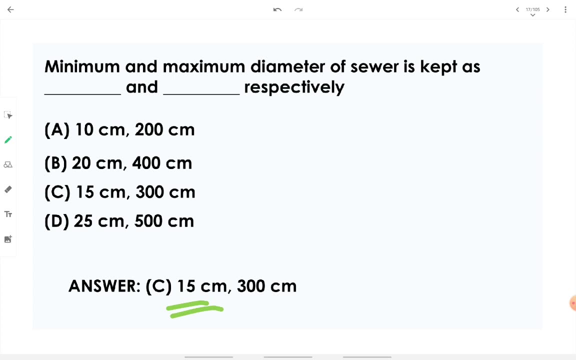 OK, design, construction and carriage of or transportation or laying of egg shaped sewer is difficult. OK, but in combined system we go with egg shaped sewer. Then minimum and maximum diameter of sewer is kept as 15 centimeter to 300 centimeter. OK, it is the range for sewer diameter: 15 centimeter to 300 centimeter. OK, remember it. Then complete the sequence for layout of a sewer. OK, So we set out, then we have the alignment and gradient set, Then we carry out the excavation with respect to the alignment and gradient. 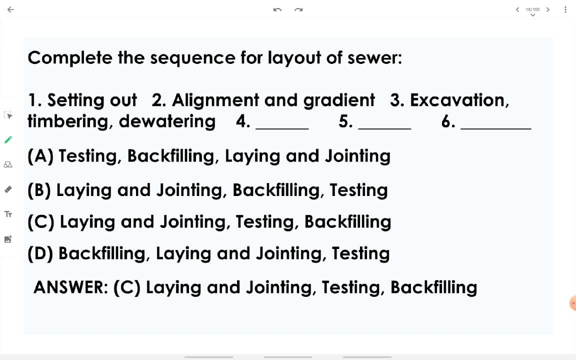 Then timbering is done, Dewatering of the trench is done, Then we lay the sewer. Then we carry out the joining process, Then we test the sewer whether they are having any leak, any crack or any gap in the joints or in the sewer itself. 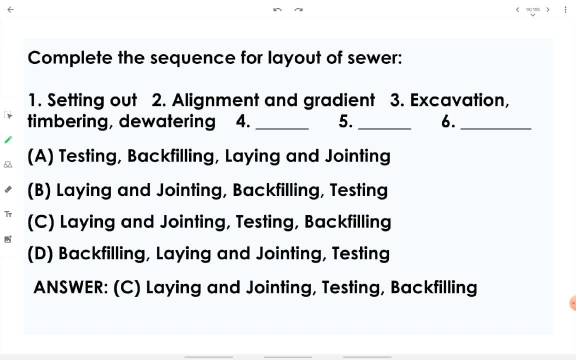 Then we fill up the sewer layout completely with the soil which was excavated first. Therefore, option C Depends the correct sequence in layout of sewer. OK, setting out alignment and gradient: excavation, timbering, dewatering, laying the sewer. 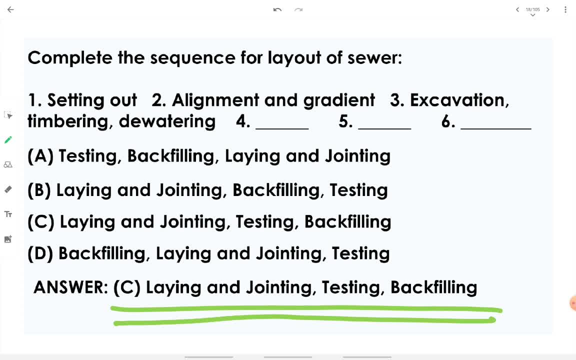 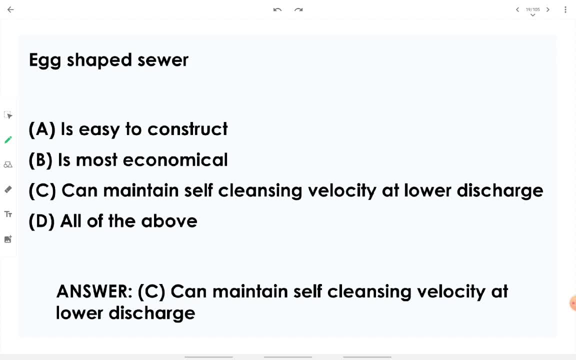 joining the sewer, then test it. then complete test is done. when complete testing is done Then we go with back filling. Then egg shaped sewer is easy to construct. No, egg shaped sewers construction is difficult. It is not economical. The initial budget involved in egg shaped sewer laying and procuring them is more. 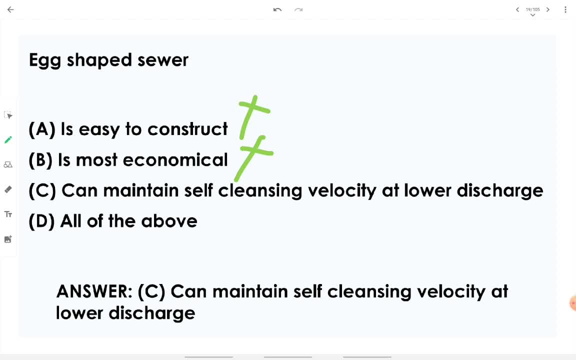 OK, it is not economical. It can maintain self-cleansing velocity at lower discharge because of the shape speciality of egg shaped sewer. the lower portion ensures that even at low discharge self-cleansing of the sewer takes place. OK, therefore, only option C is the correct choice here. 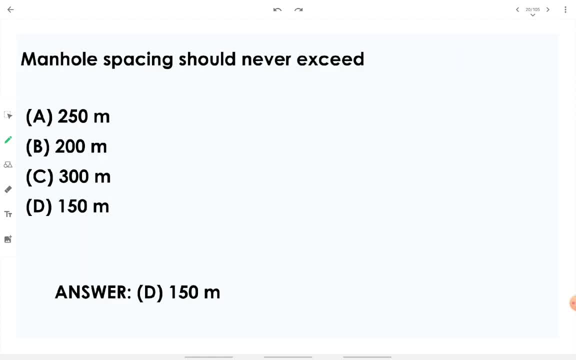 OK. answer is option C. Then manhole spacing should never exceed 150 meter. For example, let's say this sewer layout is like this: Then first manhole is there, second manhole is there. This specific distance in between the manhole should never exceed 150 meter. 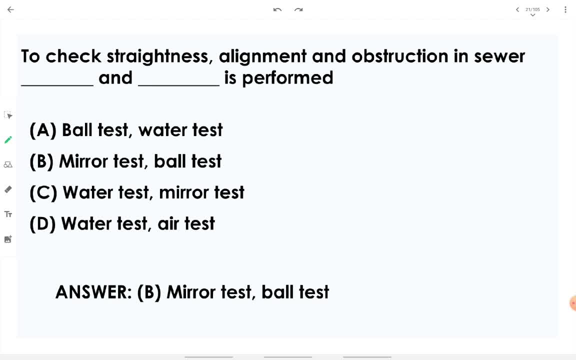 OK, Then to check straightness, alignment and obstruction in sewer, fill in the blank and fill in the blank is performed. which test we are performing? OK, we carry out straightness test: straightness by using mirror And obstruction by using ball. 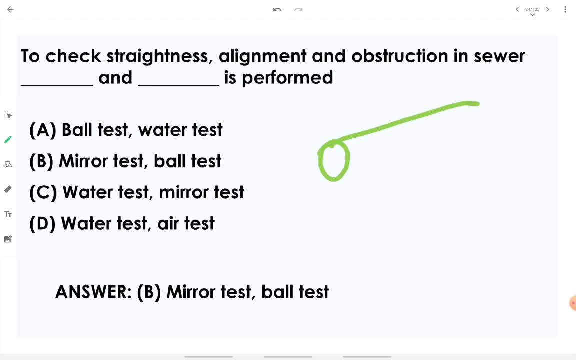 OK, in mirror test what we are doing. we are having a sewer like this. OK, then we will have a mirror and a source of light like this: OK, and the image formed by the source of light should be in one line. 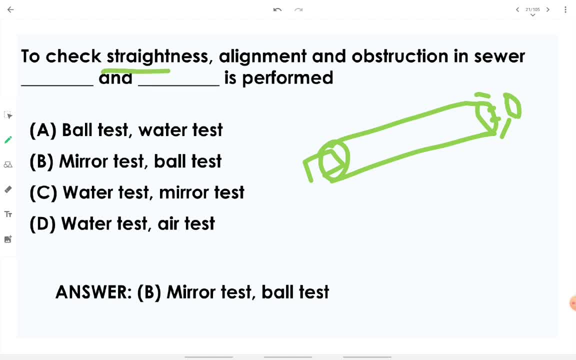 Then, and only then, we will have the confirmation of straightness of the sewer. Then, along with straightness, we are going to check alignment And for obstruction, what we will do, we will roll a ball. OK, we will roll a small ball inside the sewer. 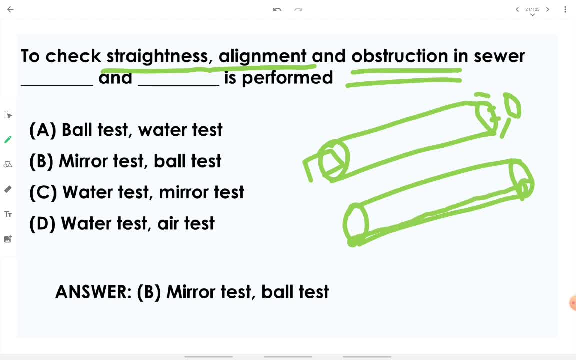 And it will keep rolling and will be collected at the other end. OK, if it is obstructing. if it is not coming out, it means that either the gradient is wrong or some obstruction is still present inside the sewer. OK, for that. what we are doing, we are getting out mirror test and ball test. 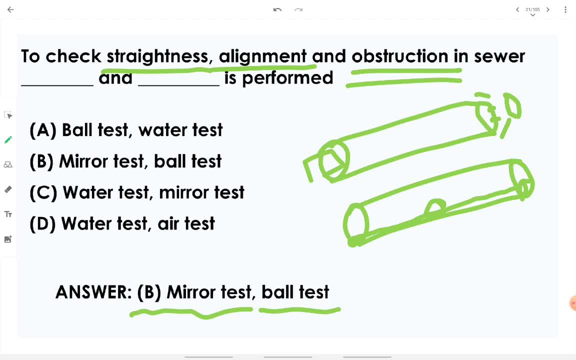 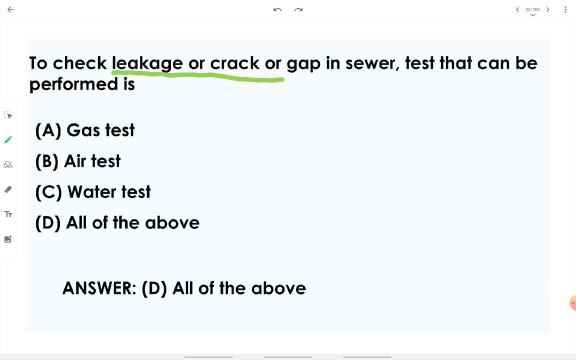 Straightness, alignment and obstruction, checked by mirror and ball. OK, water test and air test are done in order to check the joints and to check any cracks or leak inside the sewer. OK, we just saw this, we just discussed this, for checking leakage or crack or 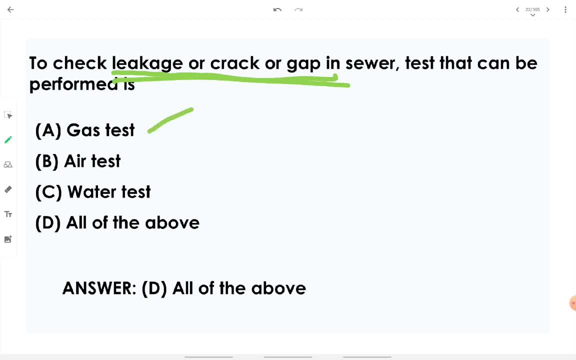 gap in sewer. we can have a gas inserted inside the sewer and exit of the gas will be checked. then it will be said that the sewer has some leak or crack or gap. OK, then air test, similar it is then water test. 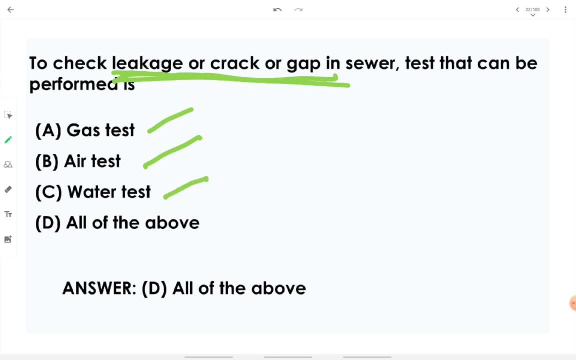 OK, water, if it is leaking from a joint, then we will make Make sure that there is leakage and we will try to repair it. OK, therefore, all of the above tests are conducted to ensure leakage or crack or gap in sewer. 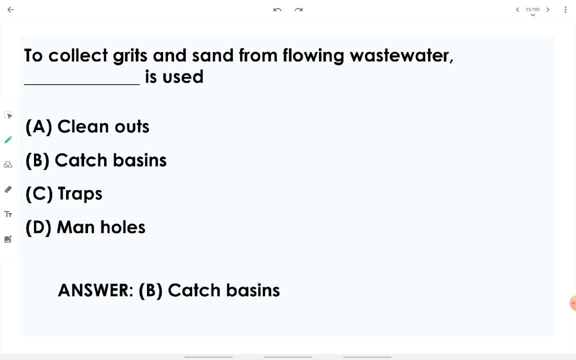 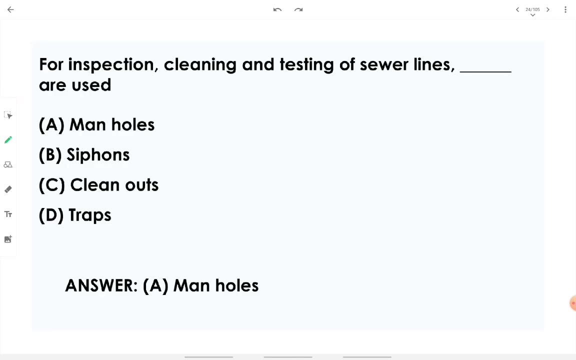 Then collect grids and sand from flowing wastewater. fill in the blanks are used. We use catch basins to collect grit and sand from flowing wastewater. Catch basins trap the grit and sand from the flowing sewage For inspection, cleaning and testing of sewer. 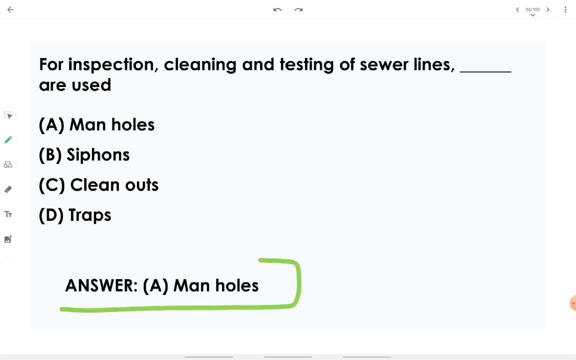 Then what we are doing? we are providing manholes over there. OK, the whole purpose of manhole is to make space for inspection, to clean the sewer line between the intervals of 150 meters and to test the sewer lines. OK, whatever the testing you want to do. 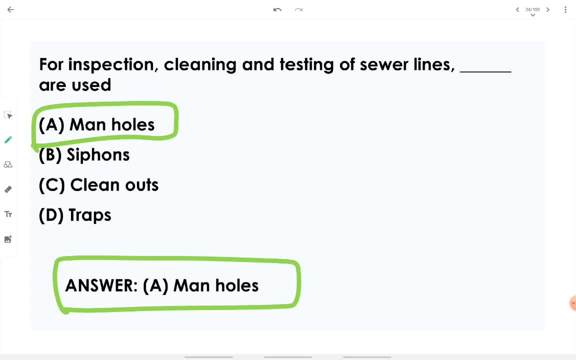 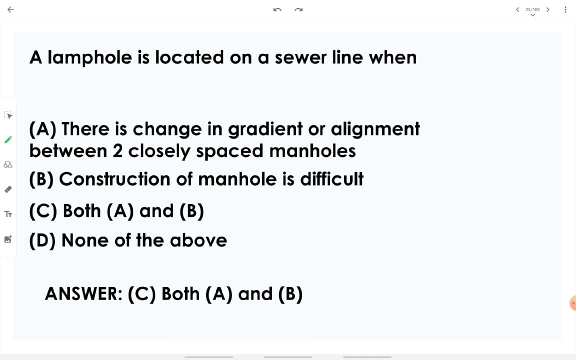 regarding sewer line, it is done by going inside the manholes. Then a lamp hole is located on a sewer line. when there is change in gradient or alignment between two closely spaced manholes, OK, if there is some gradient change, slope change or alignment change in between two closely spaced manholes. 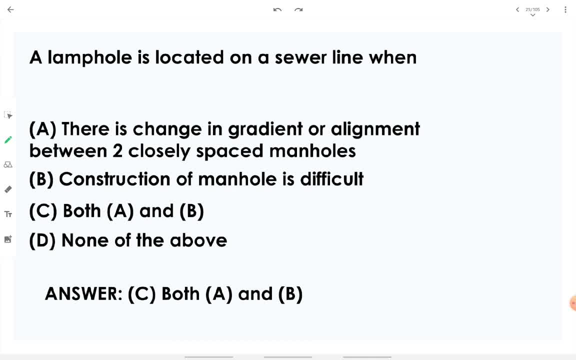 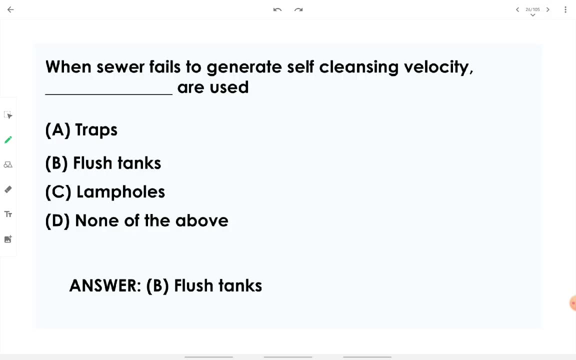 we are going to provide a lamp hole, OK, and whenever a manhole construction is getting difficult, we go with a lamp hole, OK. option C- both A and B- makes the correct answer here. Then, when a sewer fails to generate self-cleansing velocity, what we can do: 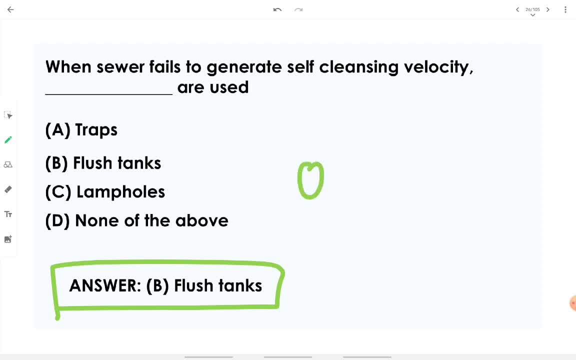 We can have the flush tanks over there. OK, what flush tank will do? Inside a sewer, let's say, if the self-cleansing velocity is not being generated, then flush tank will be there. The flush tank stores some amount of wastewater inside them and the siphoning 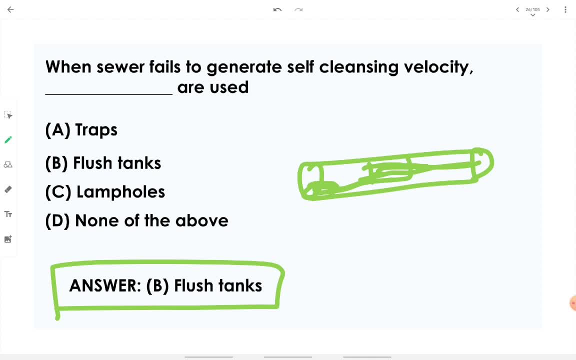 system. open the flush tank and what it will do? It will make the blockages go away. OK, suddenly, a large amount of wastewater is generated by the flush tanks. OK, it just flushes out whatever the obstacles are there present inside the sewer. 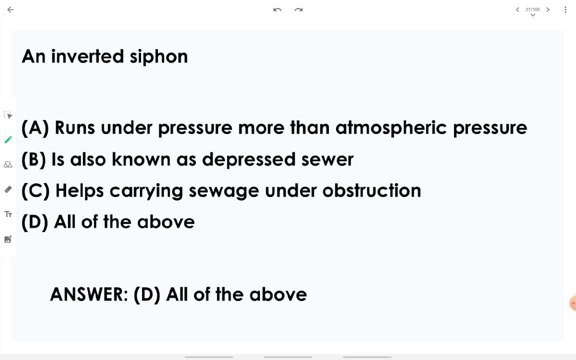 OK, what does an inverted siphon? It does run under pressure more than atmospheric pressure. Yes, correct. It is also known as a depress sewer. Yes, correct, It helps carrying sewage under obstruction. Yes, if there is an obstruction, we do provide inverted siphon which runs. 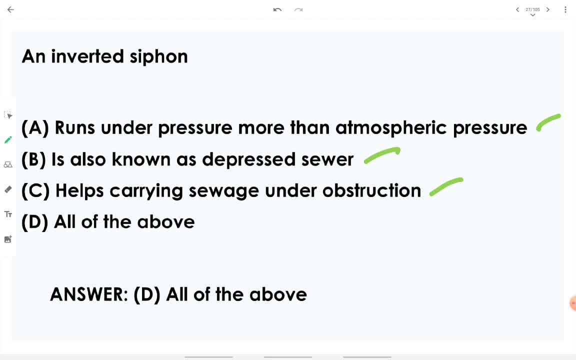 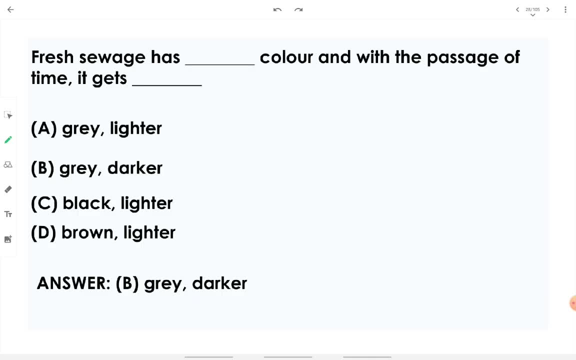 under atmospheric pressure and it is aka depress sewer. All of the above makes the correct choice. Then fresh sewage has gray color, OK. whenever fresh sewage, you will observe it is having gray color only, And with the passage of time it gets darker. 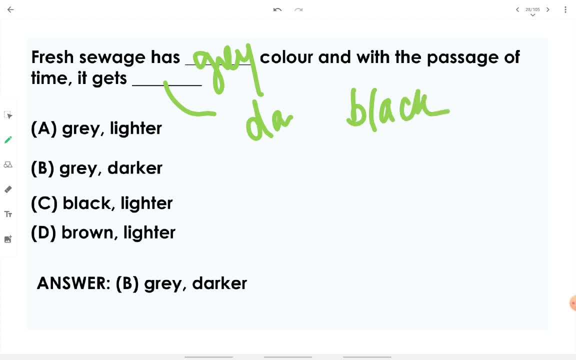 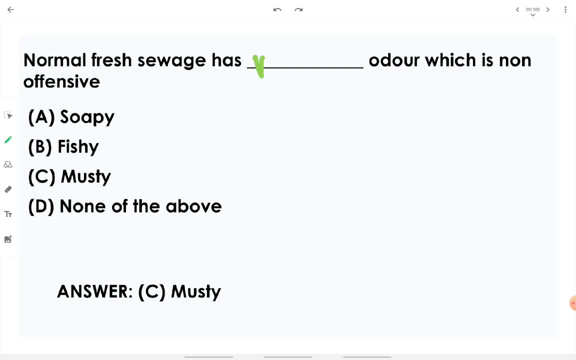 Darker means it will get kind of black colored sewage when passage of time has taken place. Normal, fresh sewage has musty order. musty It has musty order which is non offensive, which does not feel bad. OK, the order is not that much offensive. 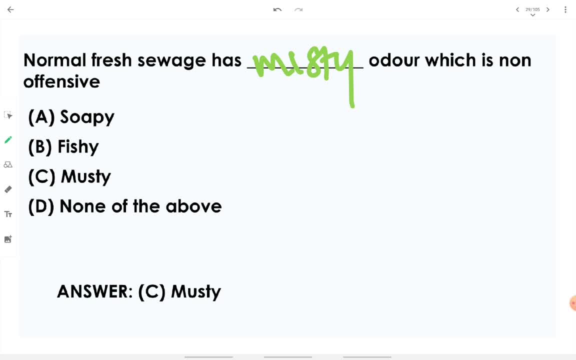 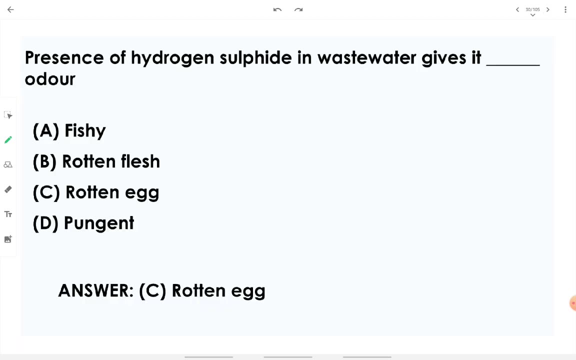 but as soon as fresh sewage has some time period passed on, when the fresh sewage is getting stale, it starts exhibiting some kind of offensive order. OK, fresh sewage has no offensive order, which is kind of musty. Then presence of hydrogen sulfide in wastewater gives it remember this rotten egg. 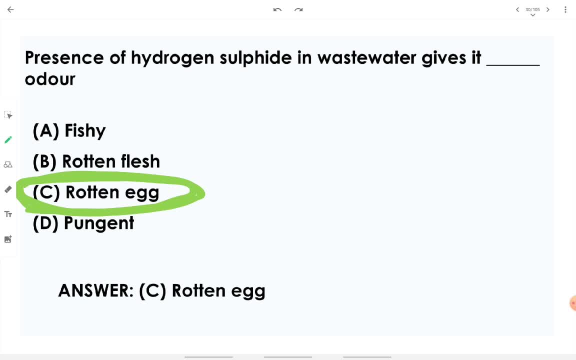 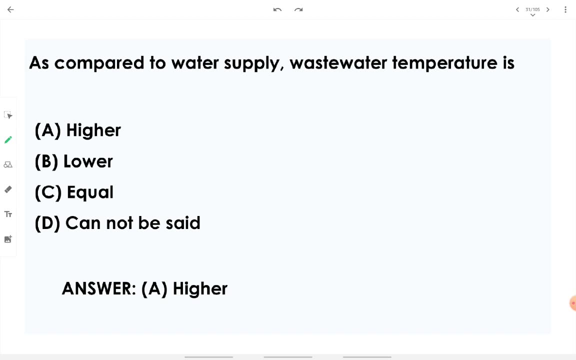 The most common question which is asked regarding a specific gas in wastewater is the hydrogen sulfide gas, which has its characteristic order, which is of rotten egg. Then, as compared to water supply, wastewater temperature is more obviously water supply temperature is lower than that of whatever wastewater temperature is there. 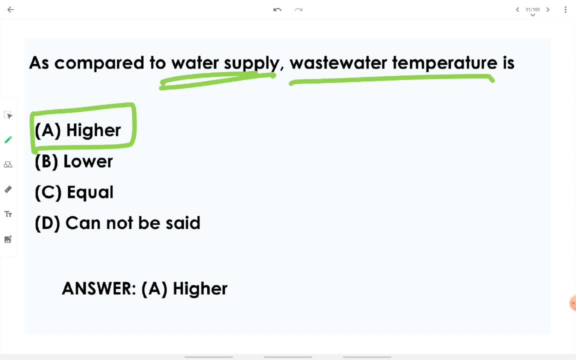 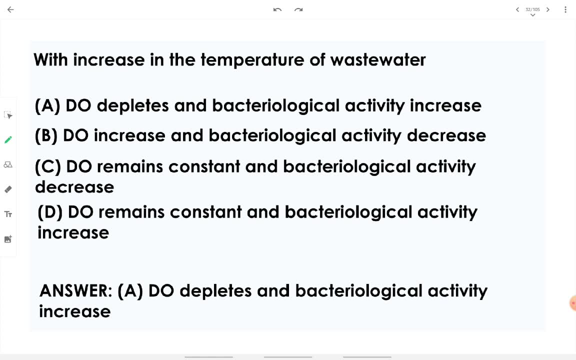 OK, wastewater will always have higher temperature. OK, with increase in the temperature of wastewater, what happens, See, when temperature of wastewater is increased? it will cause the growth of bacteria in it. OK, and as soon as the bacteria start growing, the deodepletion starts. 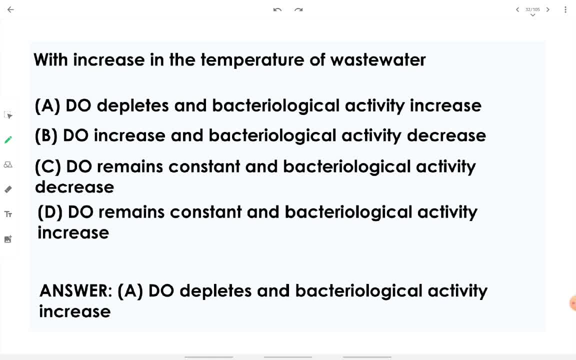 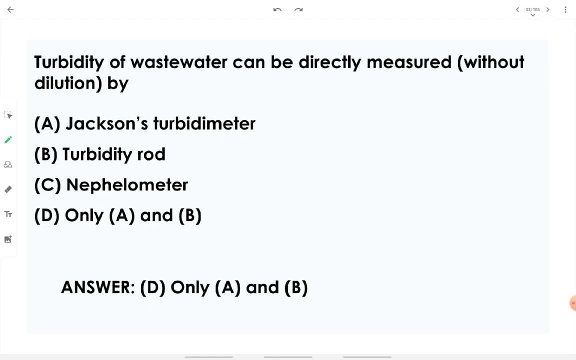 OK. therefore, with increase in temperature of wastewater, deodeplets and hydrological activity increases, Turbidity of wastewater can be directly measured. OK, directly means they are meaning without dilution- by using Jackson's turbidimeter and turbidity rod. 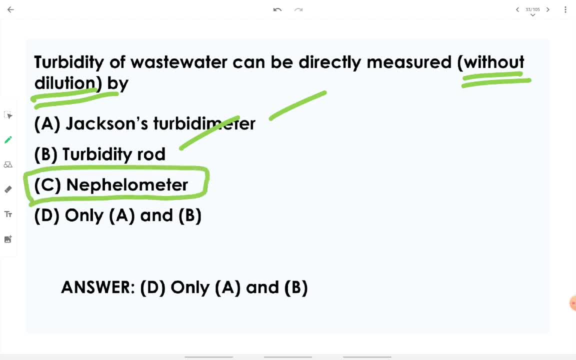 In order to check turbidity of wastewater by using a nephelometer, we have to go for some dilution- 110,, 115, whatever the dilution amount is there. We have to follow some dilution factor In Jackson turbidity meter. what we are doing, we are having the Jackson turbidimeter. 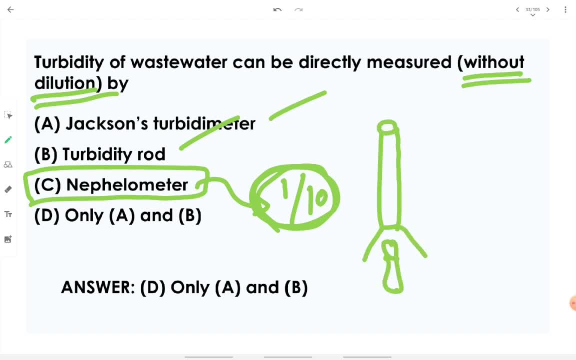 rod. then, below the rod, what we are doing, we are having a flame in form of candle or lamp. is there? OK, then we start filling the Jackson turbidity meter with wastewater. then what will happen? The flame will not be visible anymore when the column of Jackson turbidity meter is. 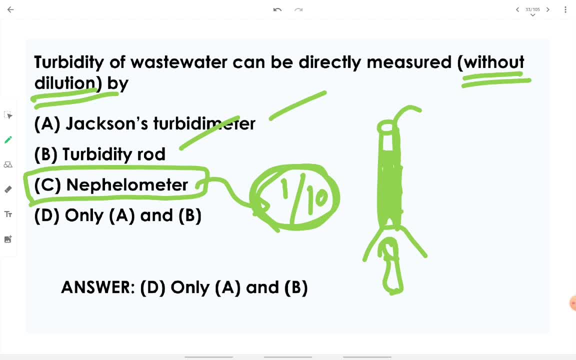 full with the wastewater. OK, if the wastewater is too much turbid, then it will take only a small amount of wastewater to make the flame invisible. OK, If pure water. if you fill it up in Jackson turbidity meter, then the flame will be still visible, because pure water has zero turbidity. 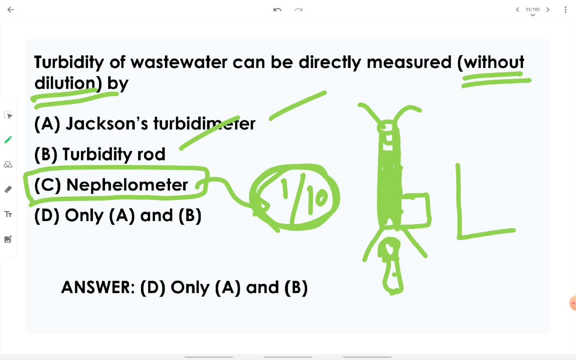 OK, Similarly, turbidity rod is used in field in order to check the how much murky or how much turbid the water sample or wastewater sample, is What we do. we get a wastewater sample which is inside the pond or can be taken out in a container. then we dip the turbidity rod inside the wastewater sample. 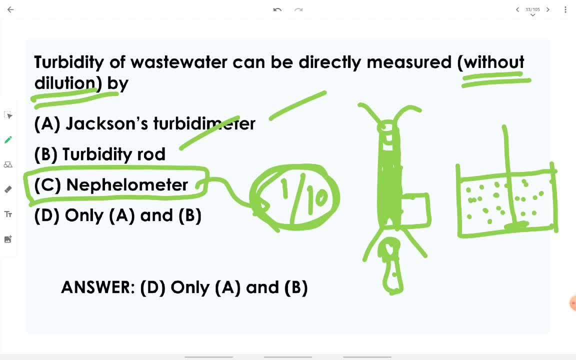 Then as soon as the very end of turbidity turbidity rod is not visible, then the graduations provided on the rod itself provide the value of turbidity. OK, if pure water, if you take as a sample and if you dip the turbidity. 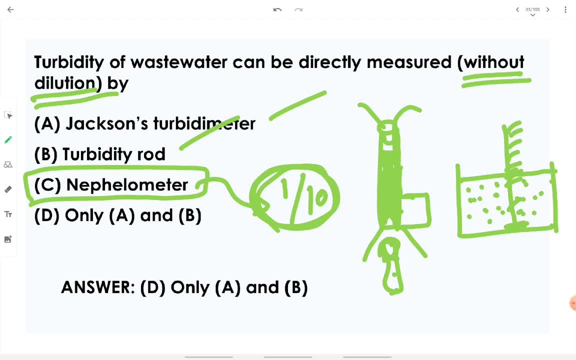 rod inside the pure water, then the rod will still be visible because pure water will not be having any turbidity. OK, depending on the strength, depending on the amount of particle present- colloidal or dissolved particle present in the wastewater- the turbidity is given. 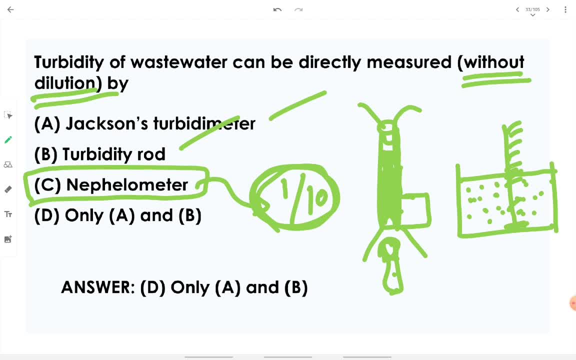 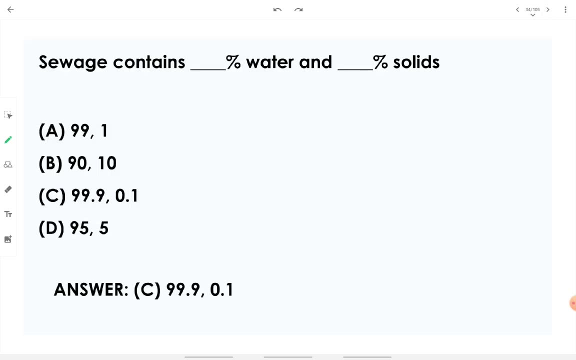 by Jackson or turbidity rod? OK, they do not require any dilution. You can directly take wastewater and use the two devices, But nephelometer does require dilution. You cannot measure wastewater directly inside nephelometer. OK, then, sewage contains 99.9% water and only 0.1% of solid. 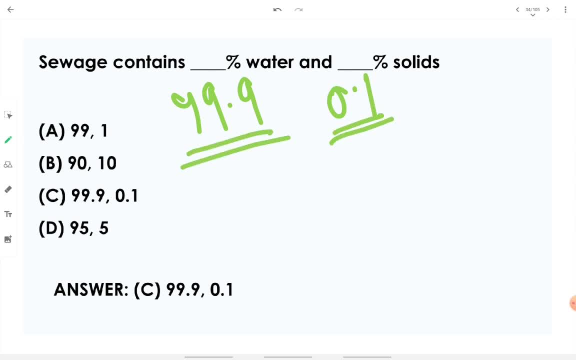 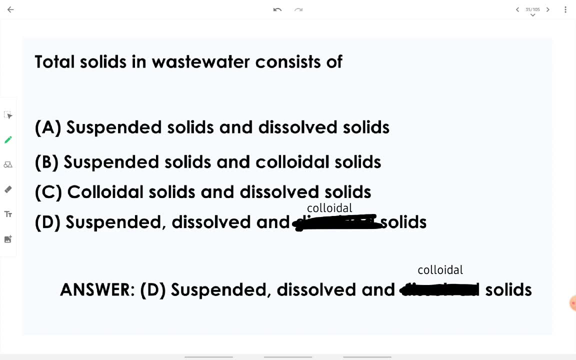 Remember this: 99.9% of water and 0.1% of solid, Then total solids in a wastewater consist of all. They do contain suspended, dissolved and colloidal solids Also. therefore, answer D, option D, is the correct answer. 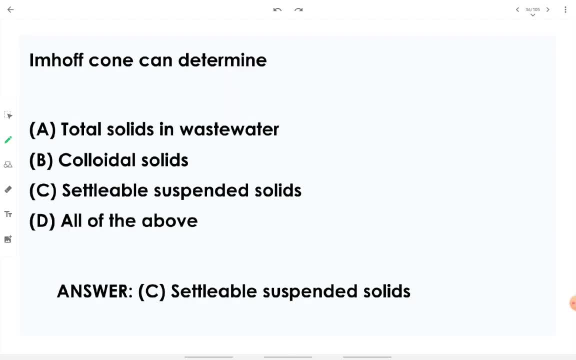 Suspended, dissolved and colloidal. Imhock cone can determine total solids, No, colloidal solids, No, they do determine settlable suspended solid, SS. settlable suspended solid are determined by Imhock cone apparatus. Then fresh sewage is alkaline in nature. 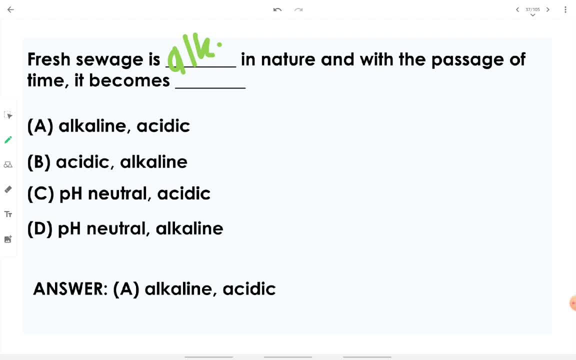 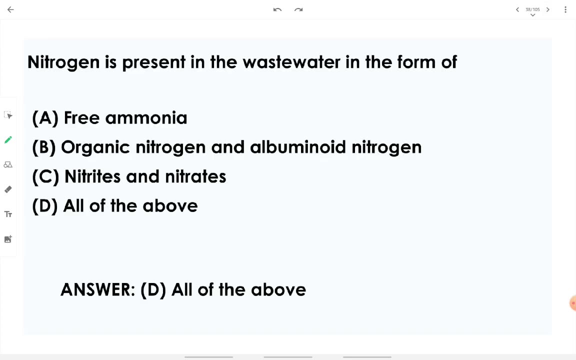 Yes, it is alkaline or basic in nature And when it gets tell, when a time passage goes by, it becomes acidic because of the reaction that takes place inside the wastewater. Then nitrogen present in the wastewater is in the form of pre-ammonia NH4 format. 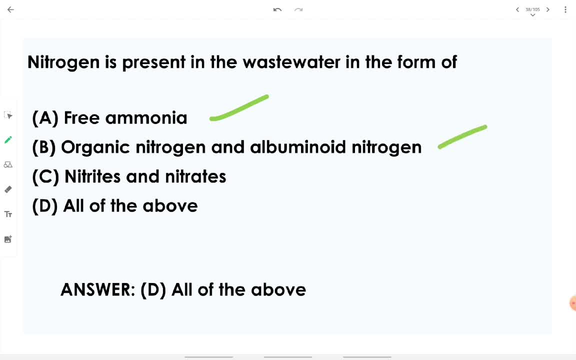 Yes, organic nitrogen, albumin and nitrogen. Yes, then nitrites and nitrates. Yes, it is present in all the format. That's why all of the above goes the right answer. OK, for aquatic life in water to sustain, the amount of DO required is 4 ppm. 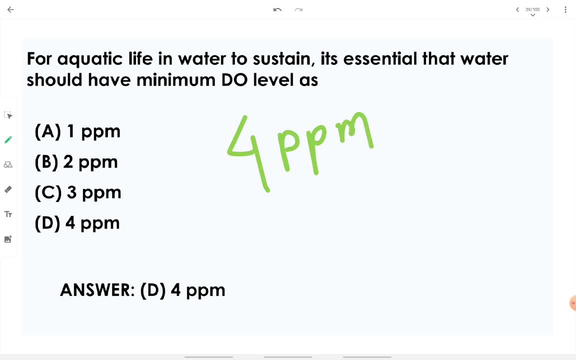 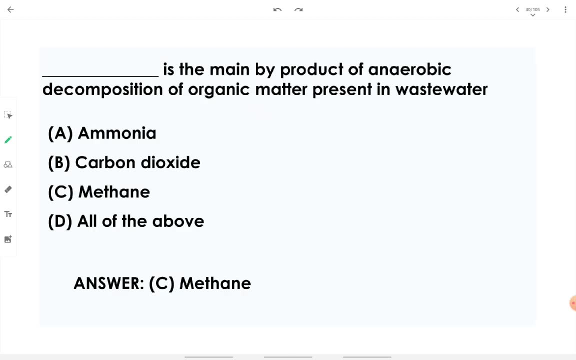 Remember it, for the flora and fauna and fish to survive inside the water, The minimum DO requirements, dissolved oxygen requirements are 4 ppm. Then fill in the blank. This is like the main product of anaerobic decomposition of organic matter present in wastewater. 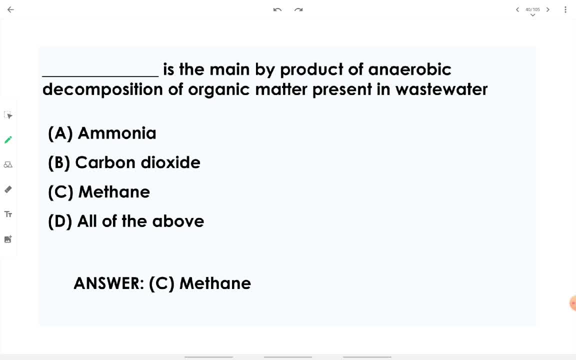 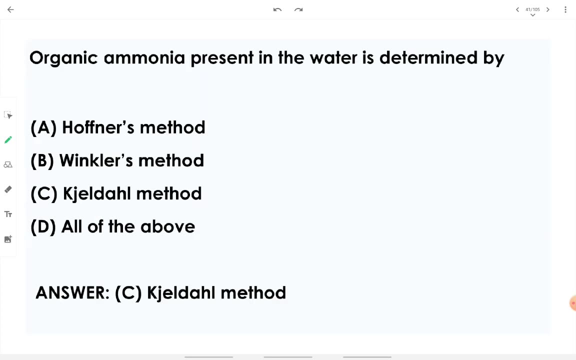 OK, when you are decomposing the anaerobic, when you are decomposing the organic matter in anaerobic way in absence of oxygen, the very byproduct that comes out of it is CH4, which is methane. OK, let's go to question number next. 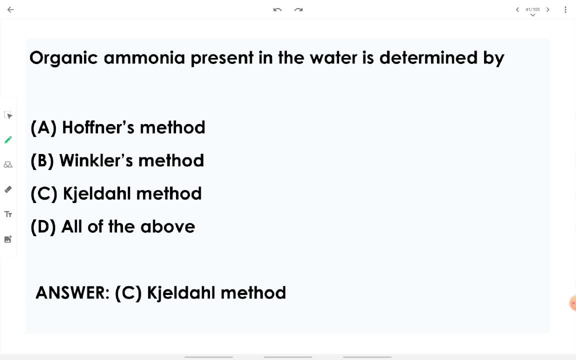 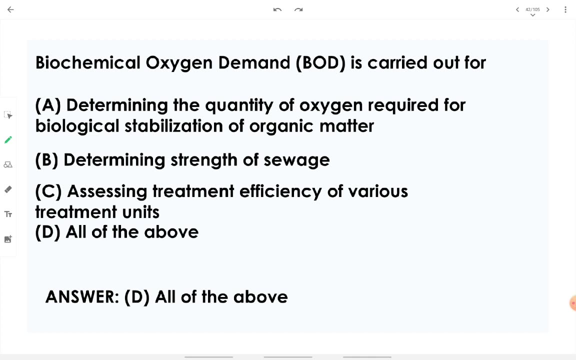 Organic ammonia in the water is determined by Gel-Dahl method. OK, Winkler's method is for DO. OK, Hoffner method is not there. OK, therefore, Gel-Dahl method is the correct answer. OK, BOD, why we are carrying out BOD. 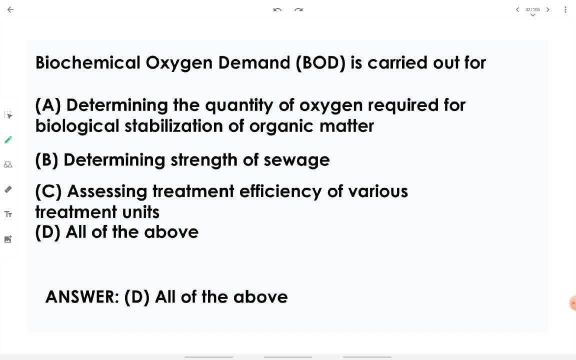 Yes, BOD is carried out in order to understand the quantity of oxygen required for biological stabilization or decomposition of organic matter. Option A is right, Determining the strength of CO2.. Yes, it is also right: Means more the BOD or more the BOD value. 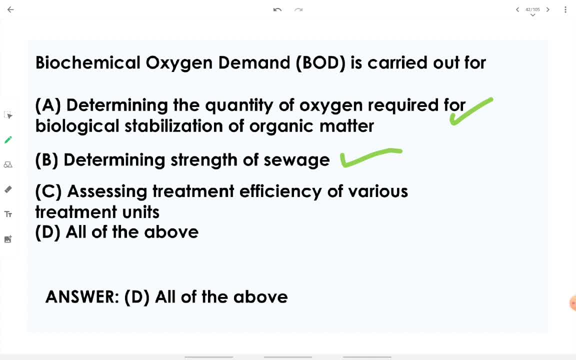 of sewage, then more its strength, more the organic matter is present in it. OK, then, to assess the treatment efficiency of various treatment units. Yes, before, after test of BOD are done. for input water BOD is assessed And for output, after the treatment unit has treated the sewage. 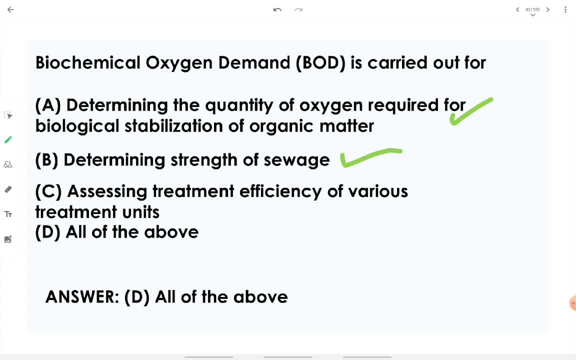 its output or effluent. BOD is tested, therefore, by the difference, more the difference, more the efficiency of treatment units. Therefore, option C is also correct. Therefore, the most correct answer goes to all of the above. OK, we are doing BOD to assess the oxygen demand. 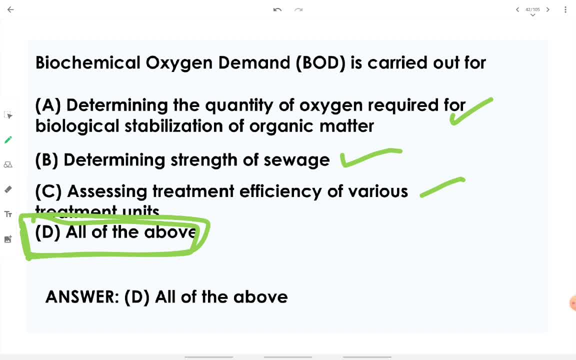 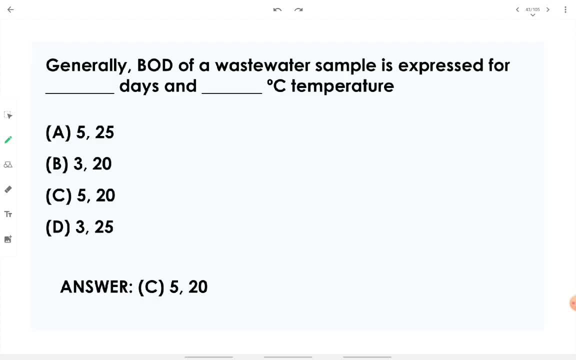 then to determine the characteristics strength of sewage and for performance analysis of treatment units Generally, BOD of wastewater sample is expressed as how many days and fill in the blank temperature. OK, see BOD 5 at direct 20 degree Celsius. 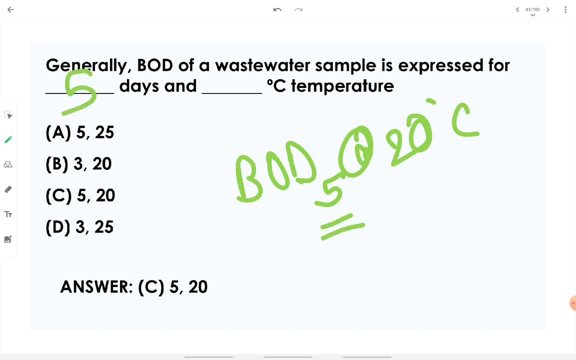 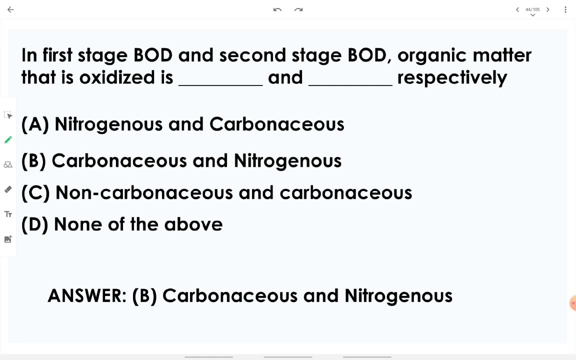 It suggests that this suffix. 5 means 5 day of BOD and 20 degree Celsius is the temperature. Option C is the one: 5 day, 20 degree Celsius BOD. Then in first stage BOD and second stage BOD- organic matter that is oxidized. 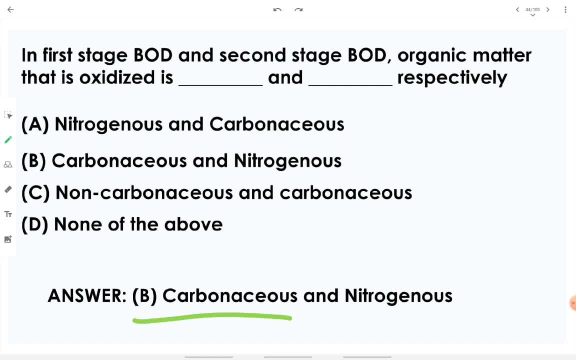 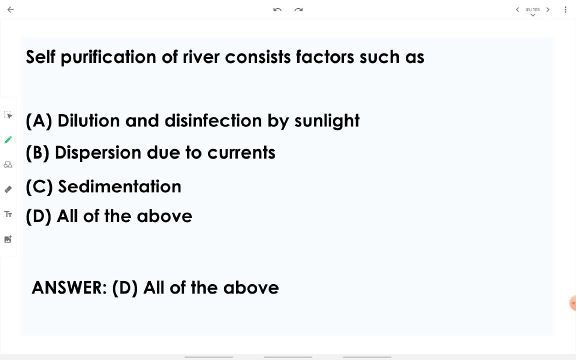 is fill in the blank and fill in the blank respectively. Always remember: carbonaceous comes first, nitrogenous comes later. OK, CN, CN is the order. OK, CN, carbonaceous first stage, nitrogenous second stage. Then. cell purification of the river consists of factors such as dilution, then disinfection by sunlight. 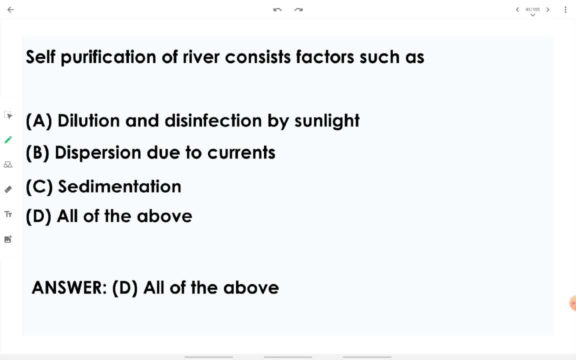 Yes, dispersion due to current- Yes, correct sedimentation because of the stream or sedimentation because of settling of the particle to the bed of the river. See what is happening when you are letting out some wastewater inside a river stream. Let's say this is a river stream which is going in this direction. 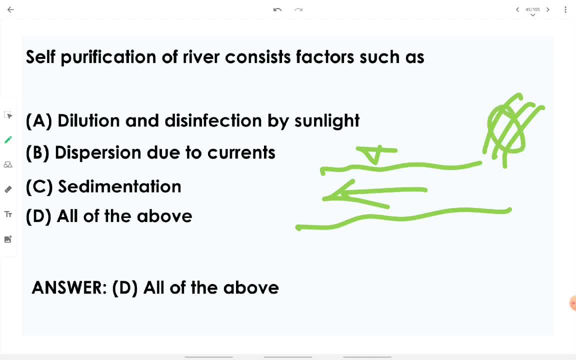 Now, when you are filling up some concentrated wastewater inside the river, it will cause dilution. OK, let's say one unit of wastewater being diluted with 500 units of water. What will happen? Dilution will obviously happen. Then sunlight is there. 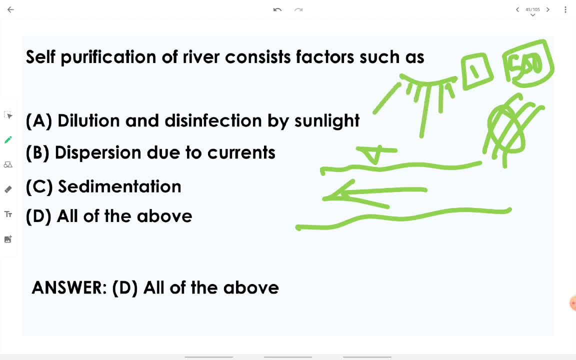 Sunlight lets out some UV rays that cause disinfection, That is, it will kill the pathogenic bacteria inside the wastewater. Then dispersion due to current. For example, some concentration of wastewater is more than the high currents- OK, high velocity current. What they will do? 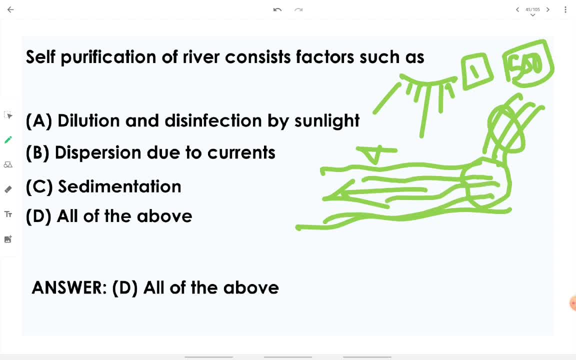 They will distribute, They will make the wastewater deeper, They will cause the equal concentration of wastewater to be distributed inside the river stream. then sedimentation- Yes, whatever the high specific gravity particle will be there, they will be settling to toward bed of the river. 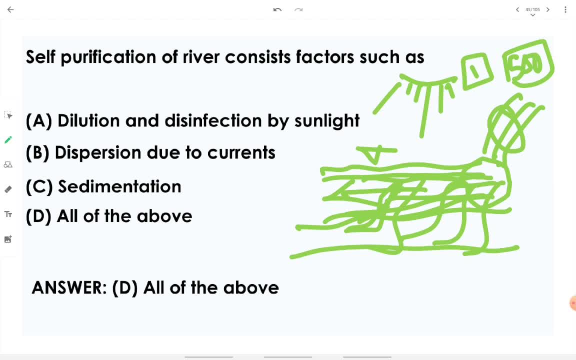 OK, and at the bed, sedimentation of the particles will take place. Therefore, the upper layer will get automatically cleans and the lower sedimented strata of organic matter will then undergo anaerobic decomposition. Therefore, the factors of self-purification of river dilution. 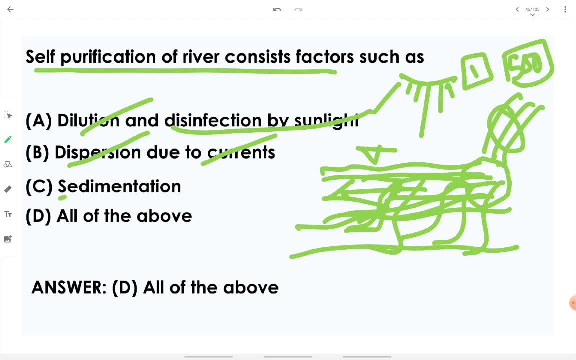 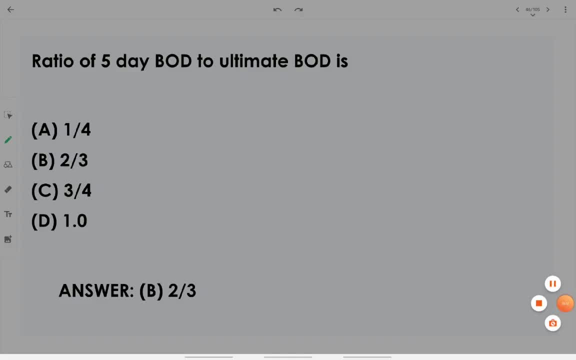 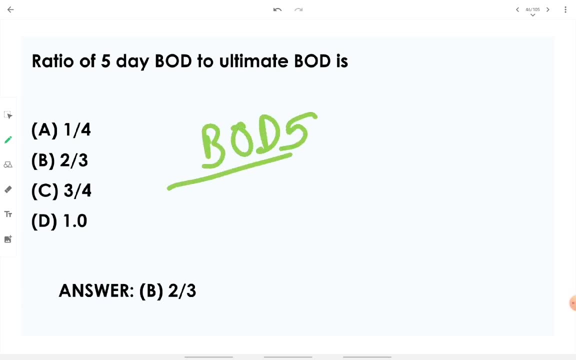 disinfection by sunlight dispersion due to strong current and sedimentation. Therefore, all of the above is the answer. Ratio of 5-day BOD to ultimate BOD is BOD5 divided by UBOD. It is always 2 by 3.. 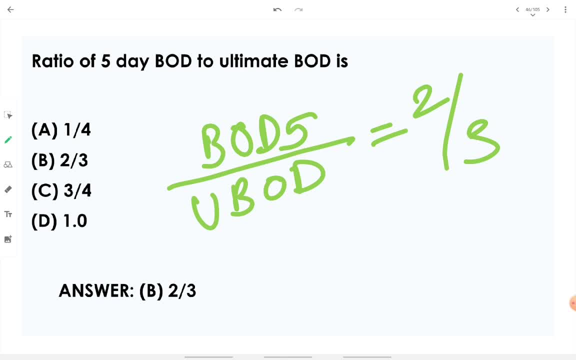 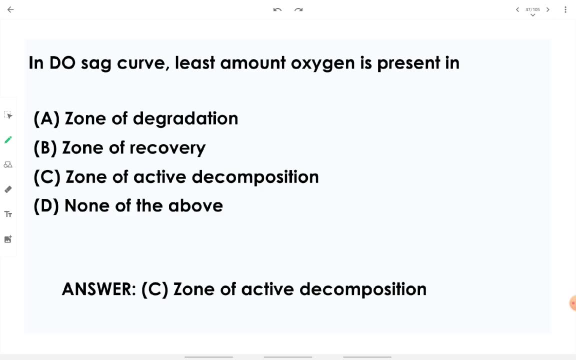 OK, BOD5 by UBOD is always 2 by 3.. B is the answer. Then in DO sag curve of a river least amount of oxygen is present in, For example, for a river which is carrying out some self-purification, or river in which wastewater is being mixed? 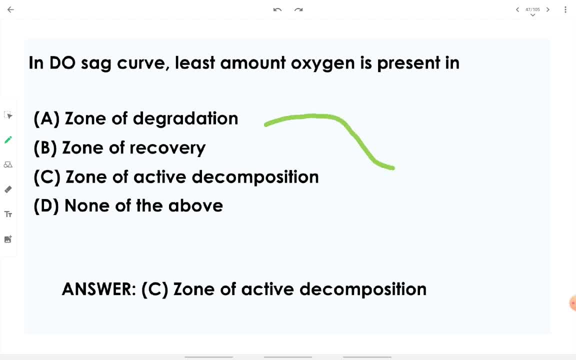 there will be a DO sag curve which is denoted something like this: OK, this is the zone of contact, First zone of contact. then this is zone of active decomposition. At active decomposition, if these are the levels of DO, let's say: 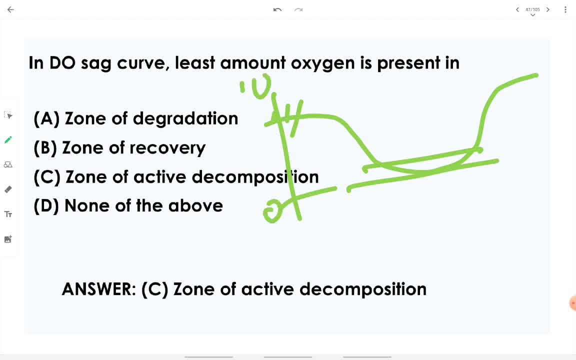 0,, 1, up to 10,, whatever it be OK. then the least oxygen is present in the zone of active decomposition, where bacteria or organic matter is getting decomposed because of action of bacteria. OK, more oxidation will take place in the zone of active decomposition. 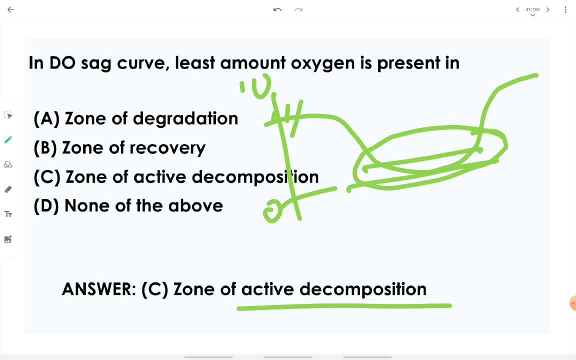 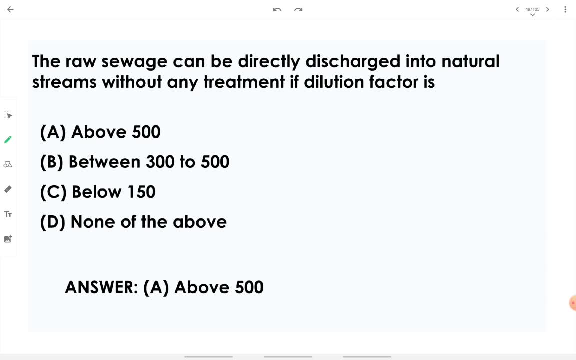 That's why all the available oxygen which is present inside the stream will get consumed. OK, therefore, it is the zone of active decomposition. Then raw sewage can be directly discharged into natural stream without any treatment if the dilution factor over there is above 500. 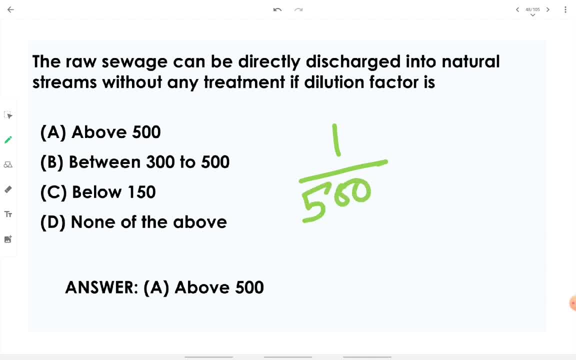 OK, therefore, the ratio should be 1 by 500.. 1 stands for wastewater unit. OK, 1 unit of wastewater, 500 for water. OK, therefore, if the ratio is below 1 by 500, if it is 1 by, 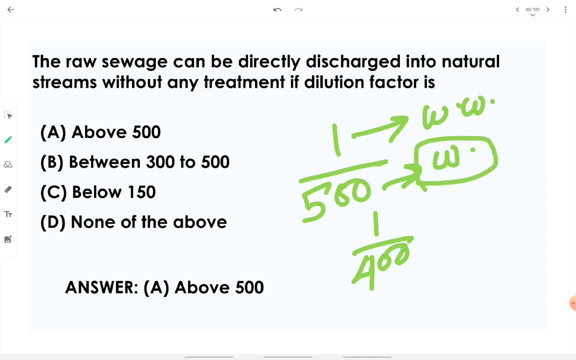 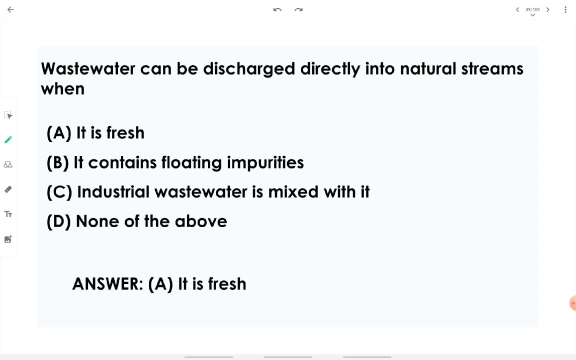 let's say 400, then less number of water units are there available for causing proper self-purification of the river. Therefore the ratio should always be kept as more than 1 by 500.. OK, wastewater can be discharged directly into natural stream when it is fresh. 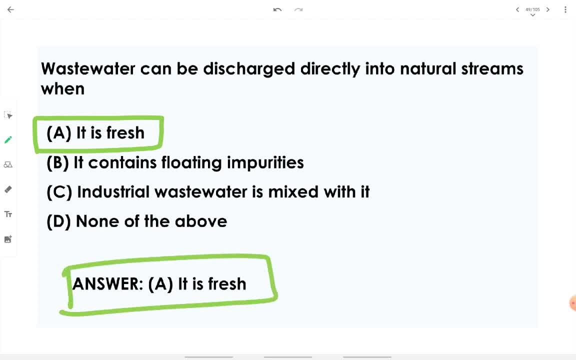 You can only dispose of the fresh wastewater. You cannot have floating impurities in it. The floating impurities must be first removed, Then the fresh water can be discharged. or if it is having industrial wastewater in it, then the inorganic impurities are so much that it cannot be treated. 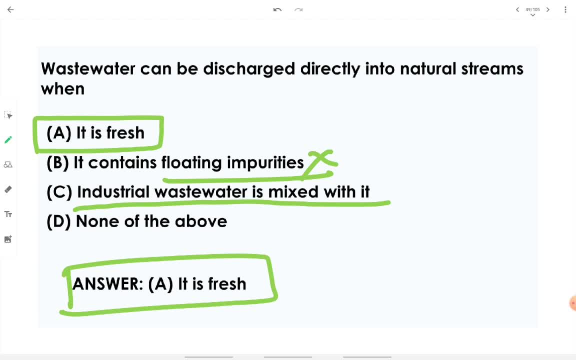 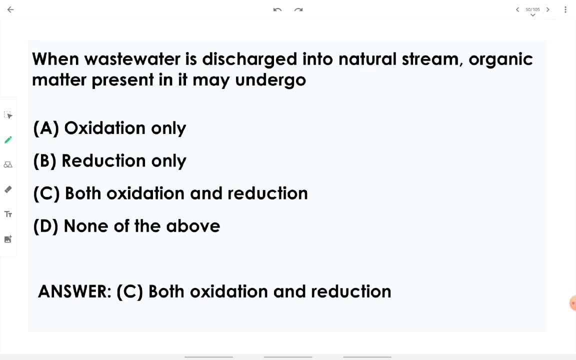 by the self-purification of stream. Therefore, we do not never let the wastewater flow into the natural water stream, which contains industrial impurities mixed with it. OK, only fresh water should be let out Then. when wastewater is discharged into natural stream, organic matter present in it may undergo oxidation as well as. 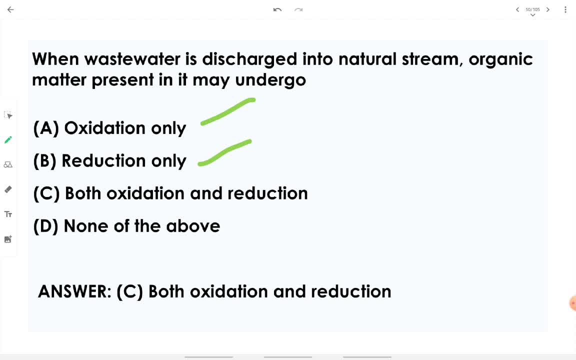 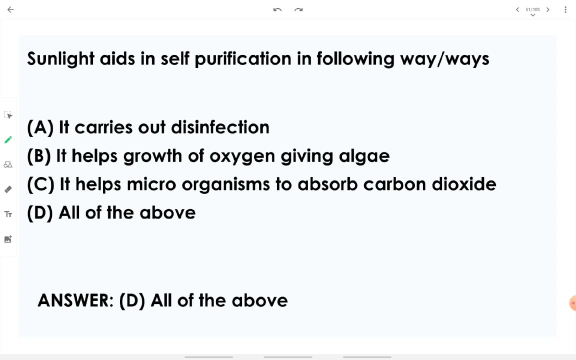 reduction OK, addition of oxygen for the composition of organic matter may take place, or removal of reduction OK or addition of hydronium ion can take place. Therefore, both oxidation and reduction processes take place. Sunlight aid in self-purification in following way or ways: 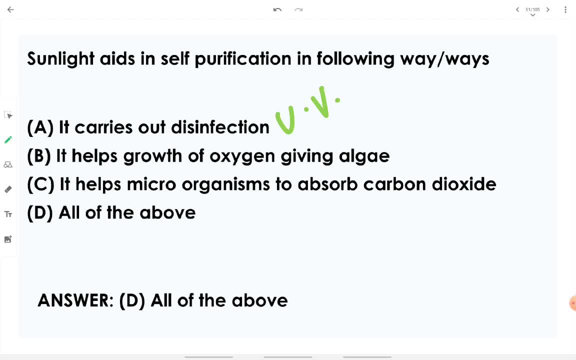 It carries out disinfection by UV rays. Yes, this is correct. It helps growth of oxygen, giving algae OK. algae need sunlight for their photosynthesis processes And while carrying out photosynthesis, they give out oxygen. That's why sunlight is indirectly helping self-purification. 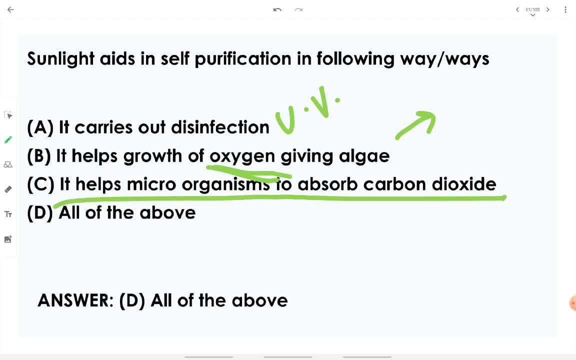 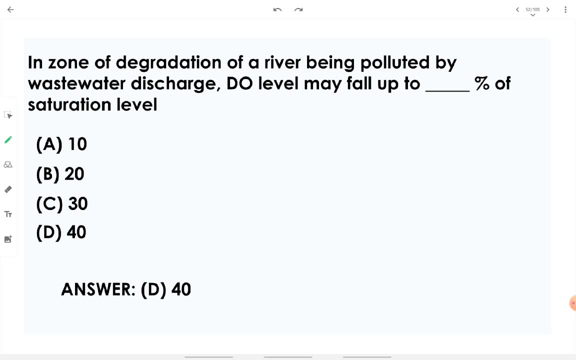 It helps the microorganism to absorb carbon dioxide. Yes, sunlight helps some specific microorganism kind to absorb the carbon dioxide which is available in the water itself. Therefore, all of the above makes the right answer for the question. Then, in zone of degradation of a river being polluted by wastewater, discharge DO level may fall up to 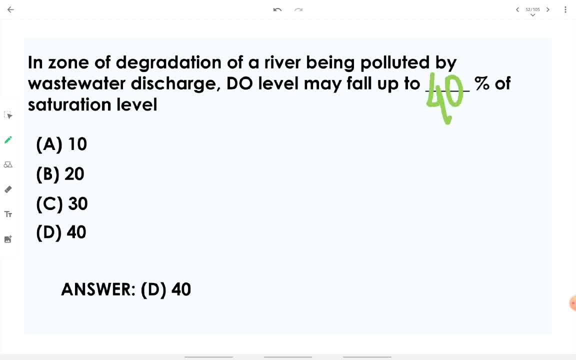 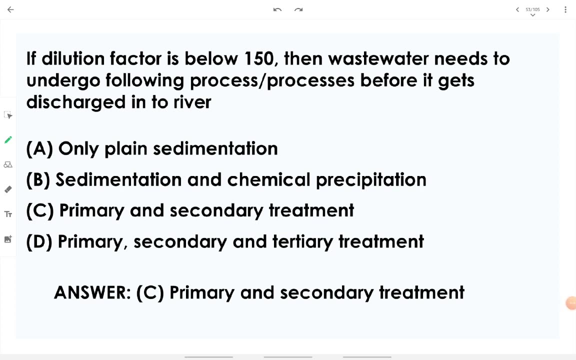 40 percent. OK, DO level fall up to 40 percent of saturation level. Whatever the saturation level for the stream is, DO level falls up to 40 percent of that. Then if dilution factor is below 150, OK, we saw the required dilution factor. 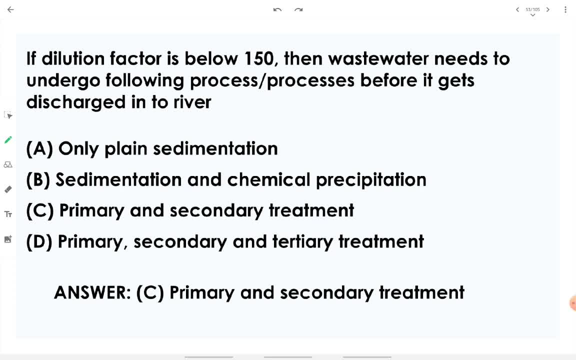 How much it should be? It should be 500 minimum. Then wastewater needs to undergo following process or processes before it gets discharged into the river: Only plain sedimentation. No Sedimentation and chemical precipitation. No Primary and secondary treatment: Yes. 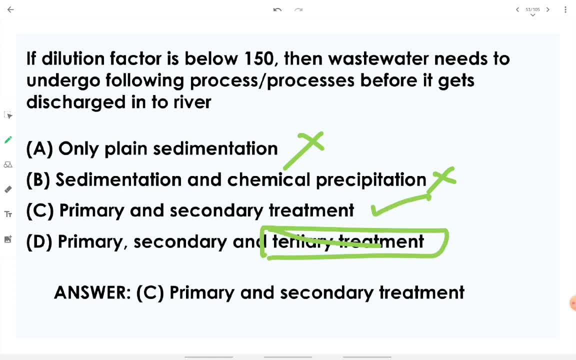 Primary, secondary and tertiary treatment. No, We do not allow tertiary treatment because it is costly and it is time consuming. OK, therefore, primary, secondary treatment is the minimum required process for allowing a wastewater to flow inside the natural river stream or natural water. 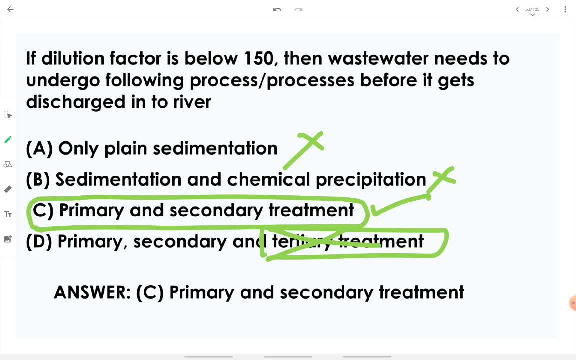 stream when dilution factor is below 150.. OK, if we are going with tertiary treatment, the wastewater need not to be disposed into what the natural river stream. You can literally separate out water and the sludge after you carry out a tertiary treatment. 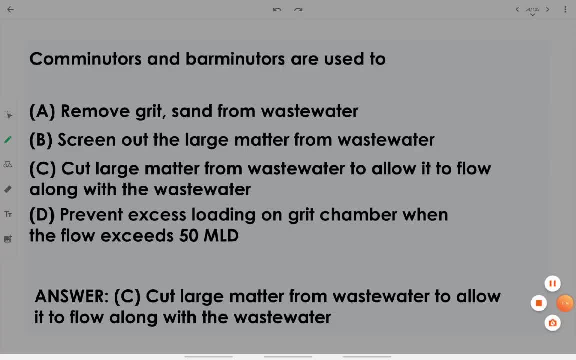 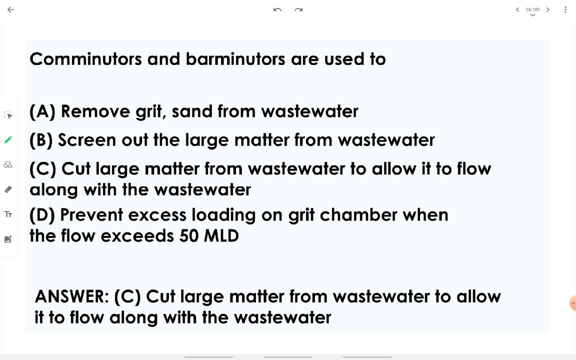 Then comminuter and barminuter are used to See. comminuter and barminuter are nothing but large size shredder that shred or that make small pieces of whatever the floating debris are coming inside the wastewater. OK, Therefore, option C: they cut out large. 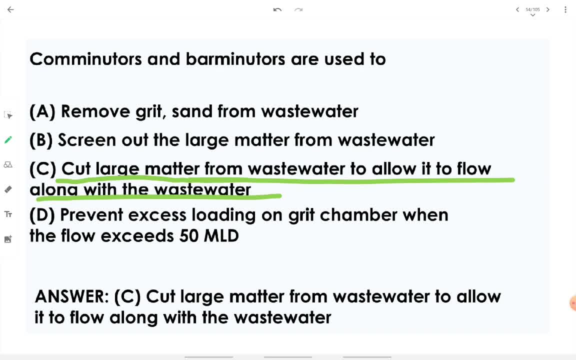 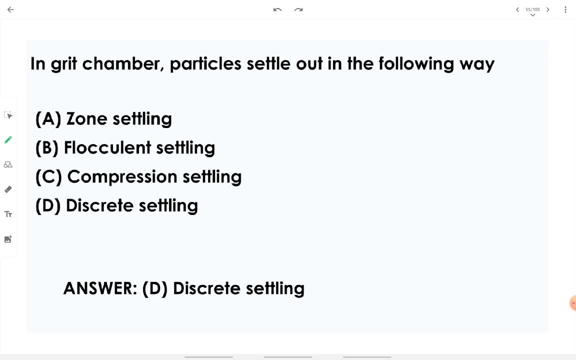 matter from wastewater and allow it to flow along with the wastewater. OK, they are nothing but shredders that carry out the shredding process In grid chamber particles set out by the discrete settling. OK, discrete settling takes place by Take place in the grid chamber so that particle can settle inside the grid chamber. 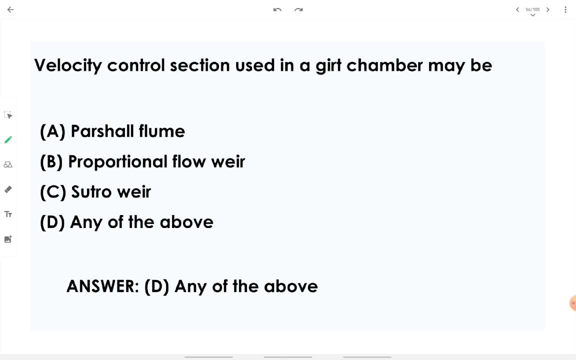 Velocity control that can be used in a grid chamber. OK, It can be a partial plume, then it can be a proportional flow wear or sutro wear. Whatever the device you want to install, you can have it, Whether it be partial plume, proportional flow wear, then sutro wear. 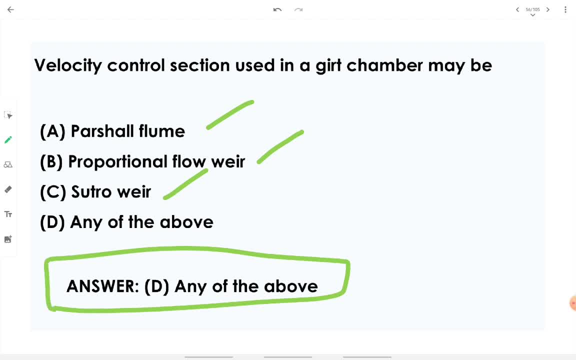 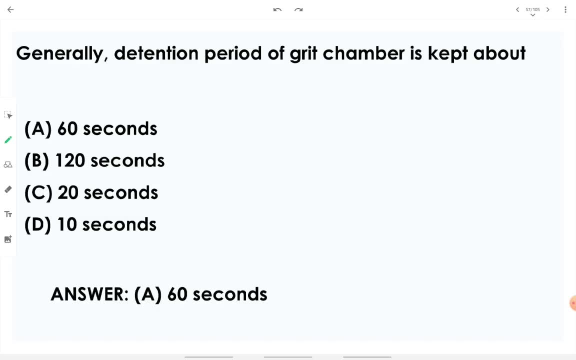 Therefore, any of the above given appurtenances can be used for velocity control in a grid chamber, not guard grid. Generally, a detention period of grid chamber is kept about one minute. OK, one minute is the detention time for grid chamber. 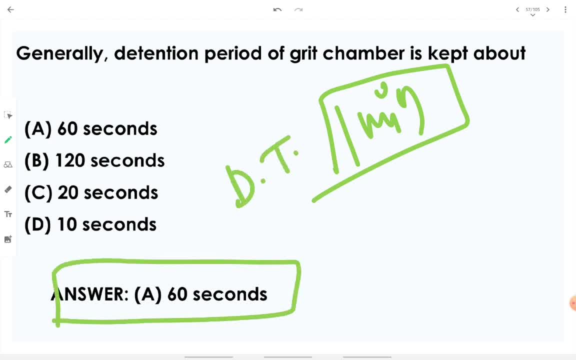 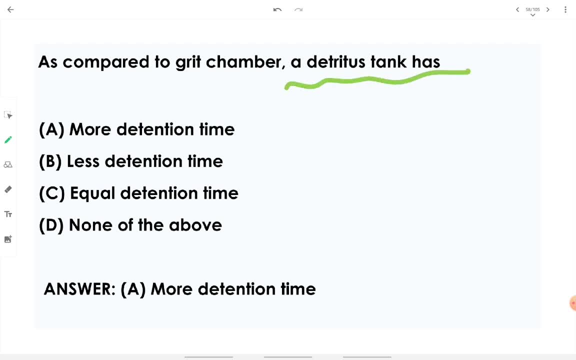 OK, which is 60 seconds. The option is correct. option is 60 seconds. As compared to grid chamber, a detritus tank has more detention time. OK, the detention time of grid chamber is generally one minute. Therefore, a detritus tank has more than one minute of detention time. 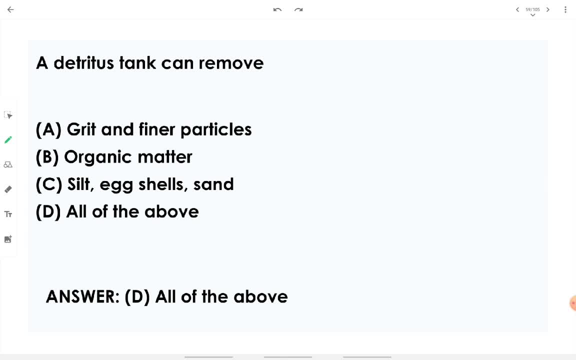 A detritus tank can remove- yes, it can remove- grit and final particle. It can remove organic matter. also, It can remove the particle with high specific gravity, such as silt, eggshell and sand. Therefore it can remove all of the above impurities mentioned in the options. 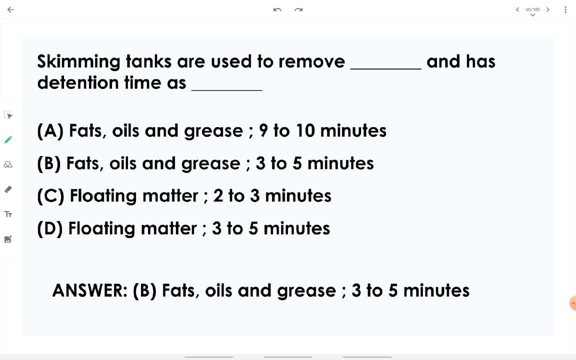 Skimming tanks are used to remove fill in the blank and have detention time. as it has DT of three to five minutes. OK, the wastewater is allowed to stay inside the skimming tank for three to five minutes. And what does a skimming tank actually do? 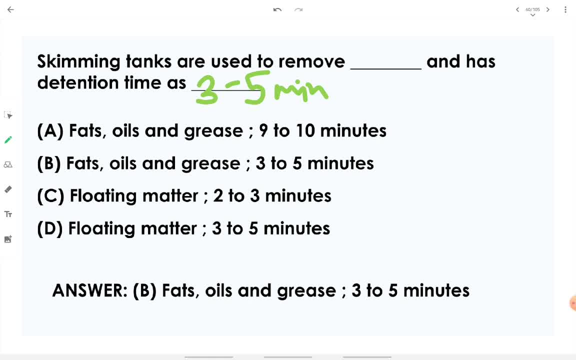 OK, it removes fats, oil and grease which are floating over the wastewater. OK, for example, let's say this is a skimming tank. Inside it a wall is provided. OK, the wastewater sets up to this level. What will happen? Whatever the fats, fatty oils or grease is there, it will go at the top layer. 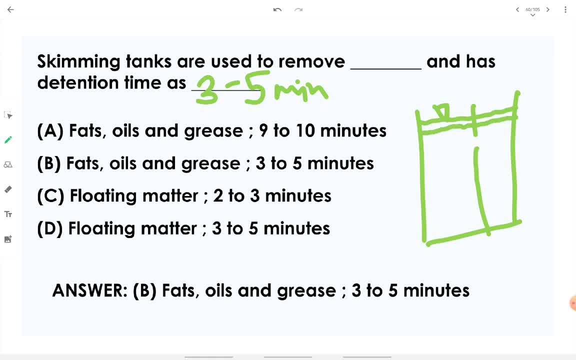 OK, therefore, whatever the remaining wastewater is there, it will. it is then allowed to pass to the next chamber. OK, the skimming action means removal of upper layer of something is called a skimming. The skimming action takes place in the upper zone of skimming tank. 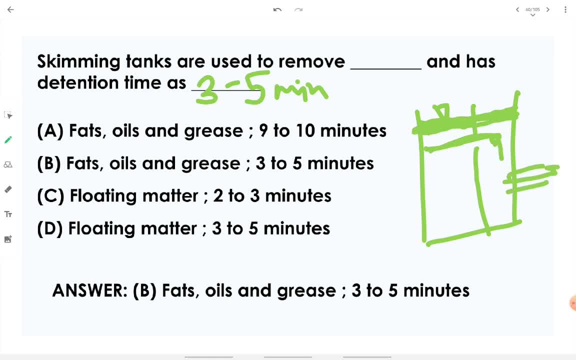 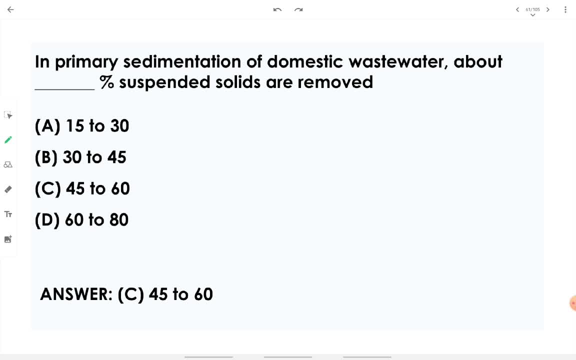 OK, and the wastewater is then sent to next treatment units. OK, in primary sedimentation of domestic wastewater about 45 to 60 percent of suspended solids are removed. OK, in PST we are aiming at removal of 45 to 60 percent. 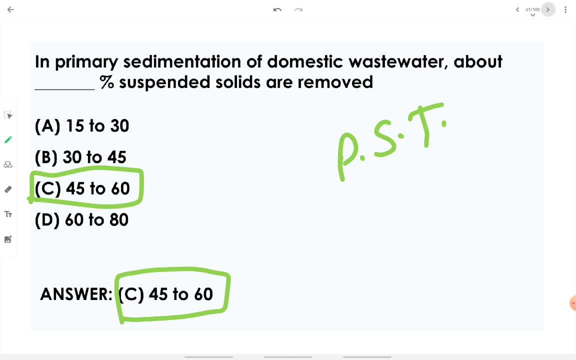 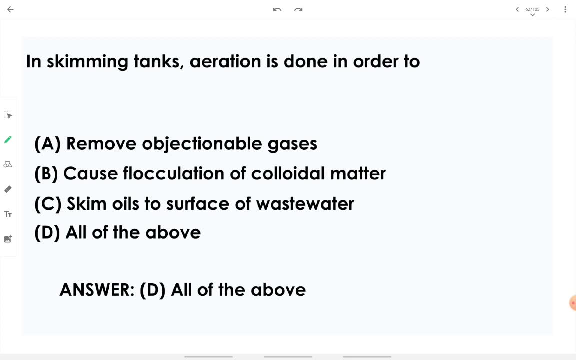 Of suspended solids 45 to 60 percent. Then in skimming tank aeration is done too. Yes, when you are providing aeration, you can get rid of objectionable gases. It then cause flocculation, flocc, formation of colloidal matter. 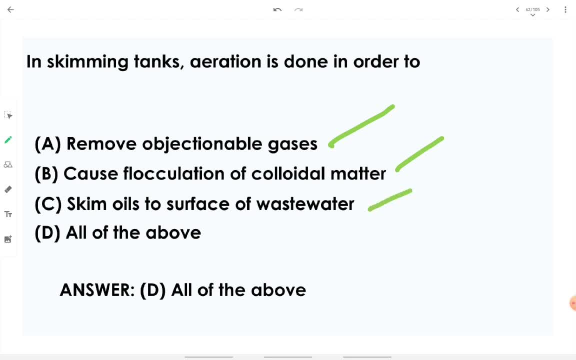 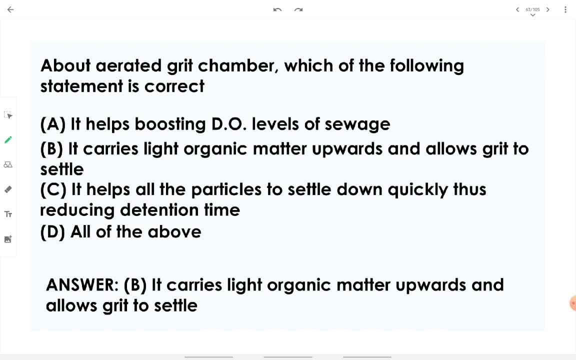 Yes, aeration causes that And it skims the oil particle to the upper surface of wastewater so that it can be skimmed easily. Therefore, all of the above actions are done by providing aeration in a skimming tank. About aerated grid chamber: which of the following statement is correct? 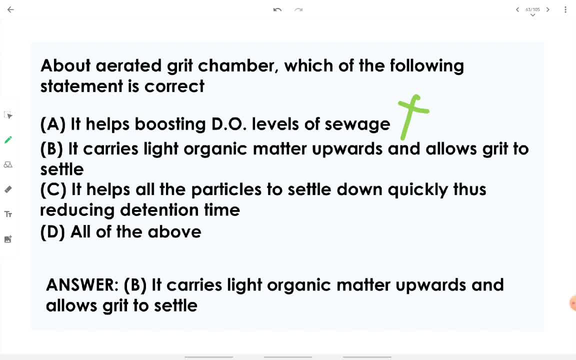 It helps boosting the DO. No, we are not aiming at DO increment at the grid chamber itself. It carries light organic matter upward and allows grid to settle. Yes, it does not allow the organic matter to settle down along with the grid, or sand or silt particle. 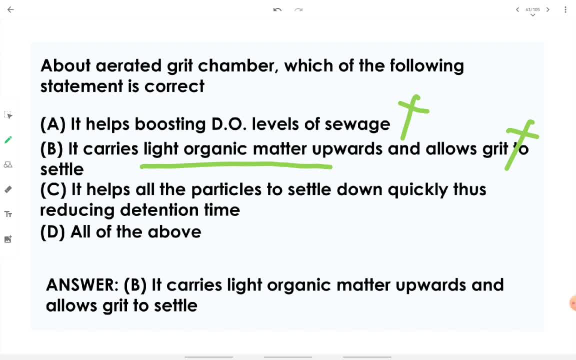 It then carries the light organic matter upward, Then it helps the particle. It helps the particle To settle down quickly, thus reducing the detention time. No, it carries light organic matter upward. and allow the grid to settle is the only motto of providing aeration in a grid chamber. 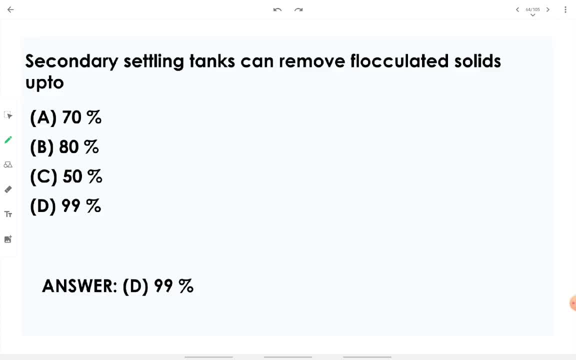 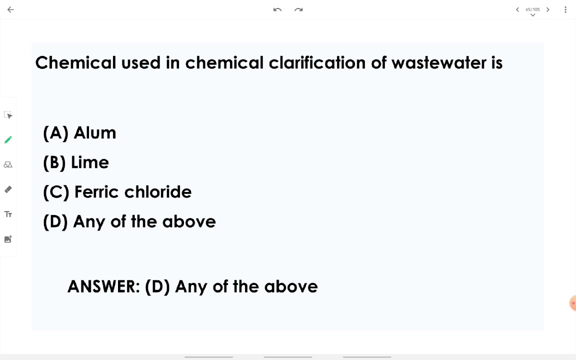 OK, option B is the correct answer. Then SST secondary settling tank can remove flocculated solids up to 99 percent. Flocculated solid in SST- 99 percent. OK, let's move on to the next question. Chemical used in chemical clarification of wastewater is alum. 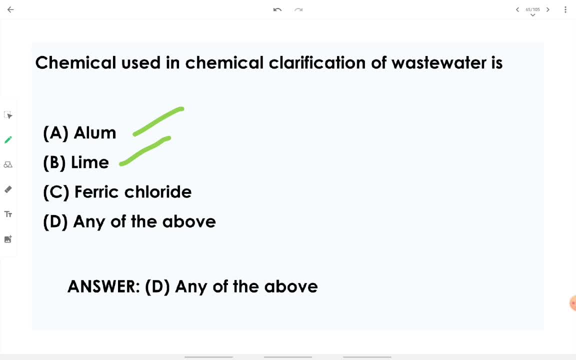 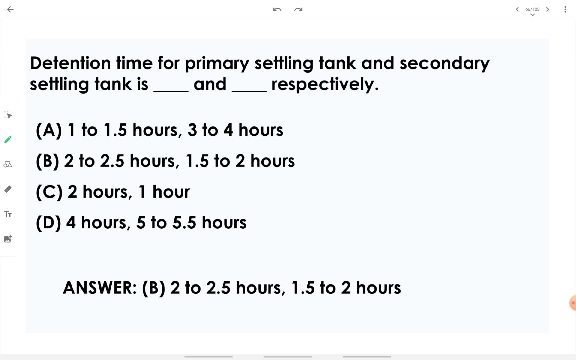 You can add alum to wastewater. You can use lime in wastewater. You can use ferric chloride in wastewater. Therefore, any of the above mentioned chemical can be used for chemical clarification of wastewater. Then detention time of PST and SST are fill in the blank and fill in the blank respectively. 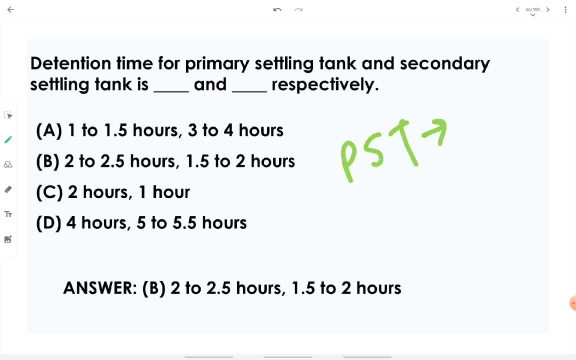 OK, remember, for PST the DT is 2 to 2.5 and for SST the detention time is lesser than that of PST, which is 1.5 to 2 hours. OK, you require more detention in primary settling and less. 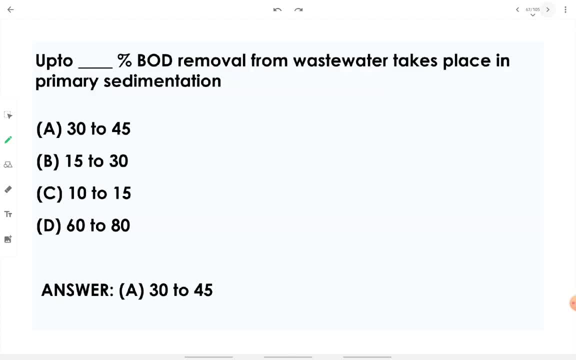 detention than that of primary settling in secondary settling tank Up to fill in the blank percent BOD removal from wastewater takes place in primary sedimentation. OK, in primary sedimentation tank we aim at 30 to 45 percent BOD removal. 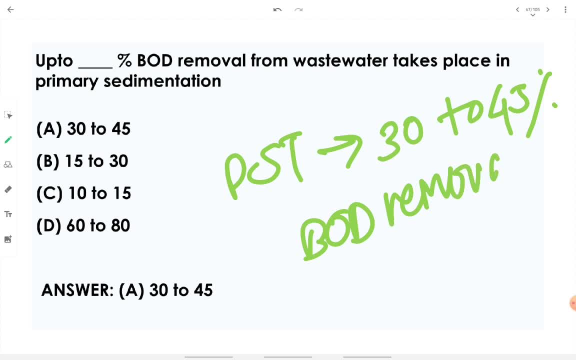 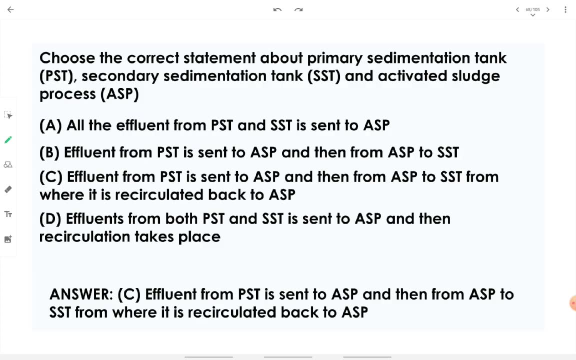 30 to 45 percent BOD removal in PST. Choose the correct statement about primary sedimentation tank, secondary sedimentation tank and ASP. OK, they are talking about flow of wastewater from PST, SST to ASPC. Let's just draw a small diagram here. 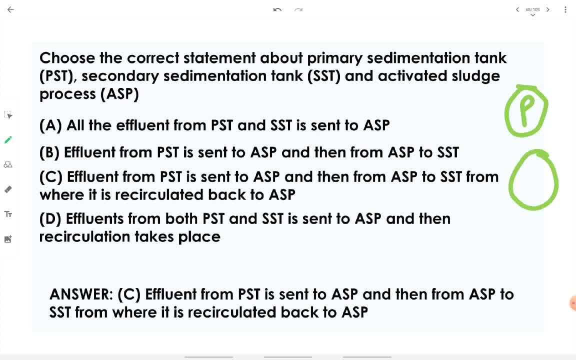 Let's say this is primary sedimentation tank. Let's say this is ASP. Let it denote by A and this is SST. OK, secondary sedimentation tank. Whatever the effluent is from PST is first sent to ASP. OK, then from ASP it goes to secondary settling tank and a portion 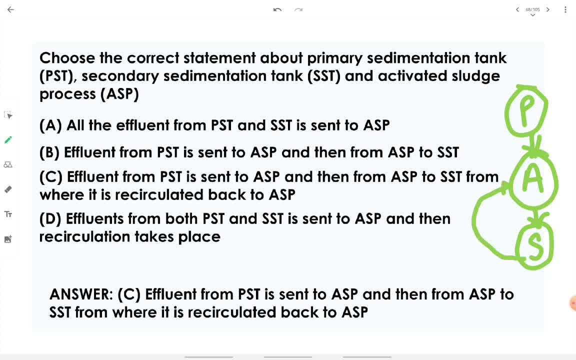 let's say 10 percent, 20 percent portion is recirculated back to ASP. OK, this is the flow diagram for effluent from PST to ASP to SST And from SST back to ASP. Therefore, effluent from PST is sent to ASP and then from ASP to SST, where it is recirculated back to ASP. 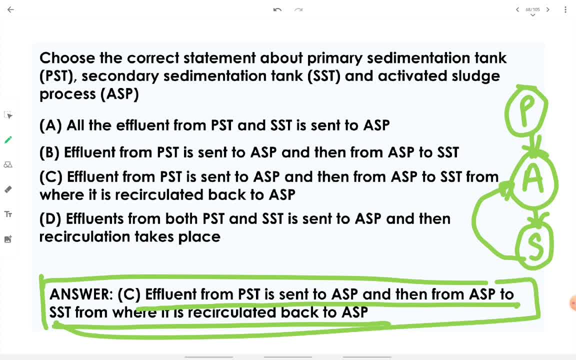 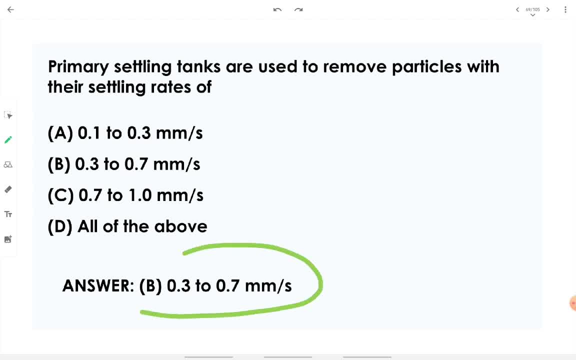 Option C is correct choice here. OK, primary settling tanks are used to remove particle, with their settling rate of 0.3 to 0.7 mm per second. OK, the settling rate of particle is 0.3 to 0.7 mm per second. 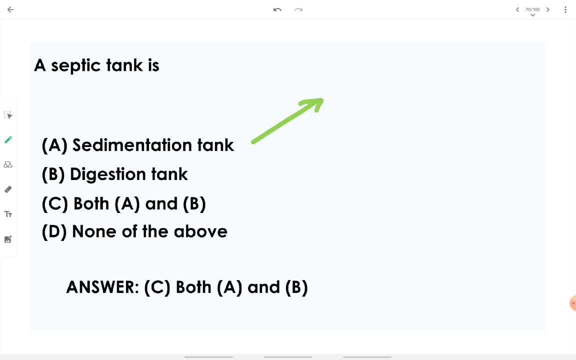 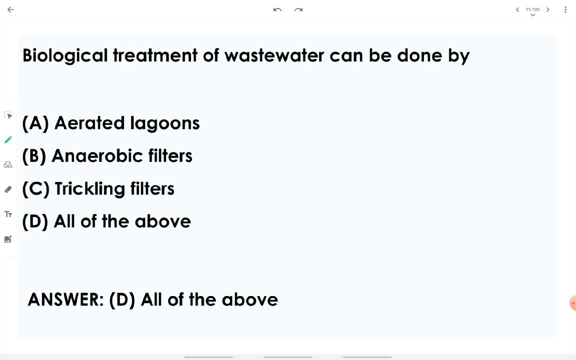 Then the septic tank is. it is a sedimentation tank. Yes, it allows the heavier particles to settle down and it carries out digestion of the settled particle. Therefore it is both sedimentation, settling and digestion tank. Then biological treatment of wastewater can be done by aerated lagoon. 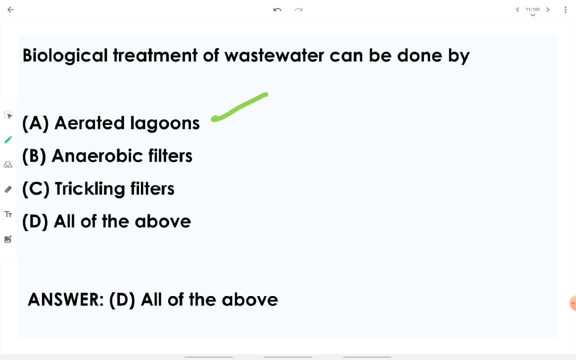 Yes, the lagoons which are continuously provided with oxygen are aerated lagoon. Anaerobic filter: Yes, they are also biological treatment where anaerobic bacteria carry out decomposition of organic matter. They are present in the wastewater by absence of, even in the absence of oxygen. 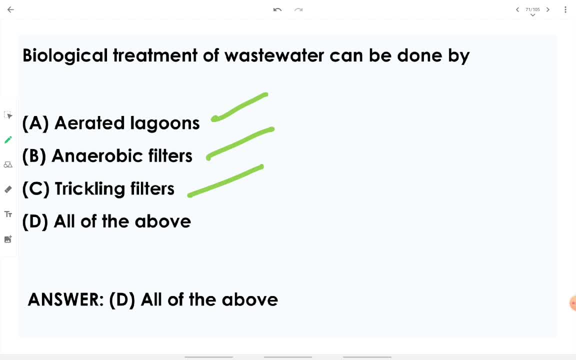 Then trickling filter. Yes, the wastewater is sprayed on the porous stone which is present inside the trickling filter, and they do carry out the decomposition by having a fixed film growth on the stones of trickling filter. Therefore, all of the above is the correct answer. 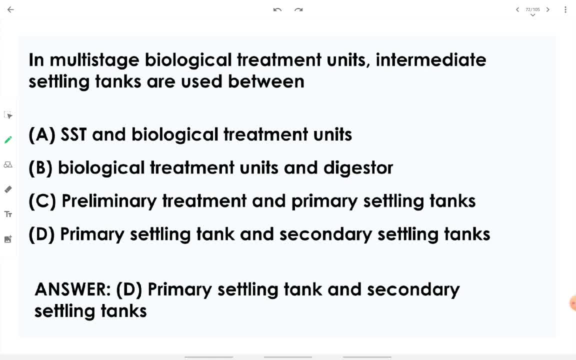 Then in multistage biological treatment units intermediate settling tanks are used between PST and SST. If the more settling is desired in the wastewater treatment facility, then in between PST and SST intermediate settling tanks are provided. Okay, if it is required. 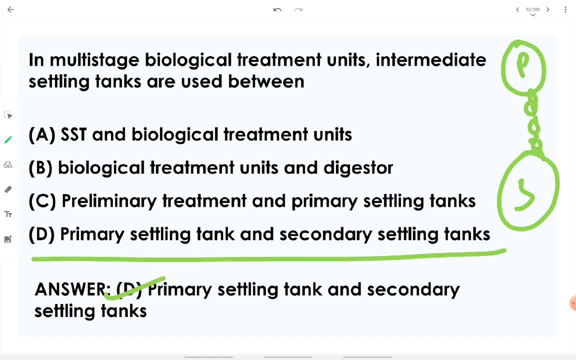 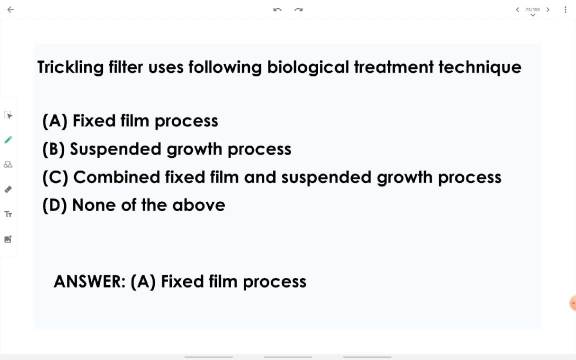 Therefore option D is correct. Trickling filter uses following biological treatment technique. Is it fixed film growth: Yes. Suspended- No. Combined: No. None of the above gets ruled out. It is fixed film process In a trickling filter. number of stones are there? 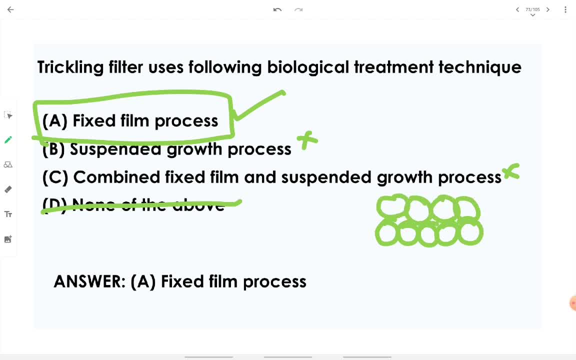 Okay number of porous stones are there and over the porous stones wastewater is continuously sprayed. and the sprayed wastewater locks inside the pores because of the organic impurities present in it. Now the impurities are blocking the minute pores inside the stone and causing more. 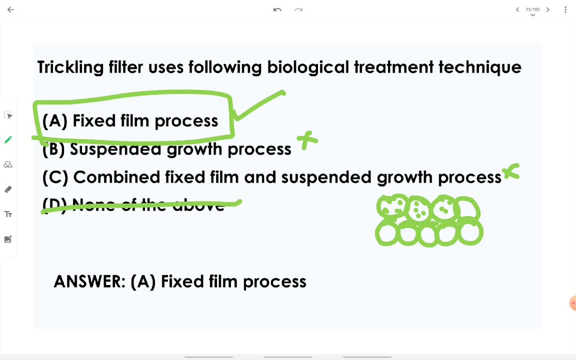 effective filtration process, and while the organic impurities are locked in the minute pores of the stone, organic growth of bacteria and the slimy growth of the organic matter takes place over the stone. And now this biofilm, which is called as a fixed film, then carries out the remaining biological treatment. 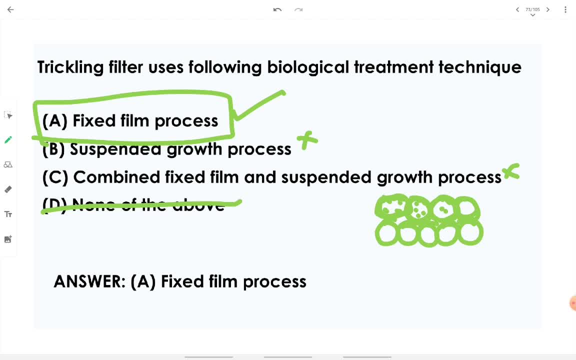 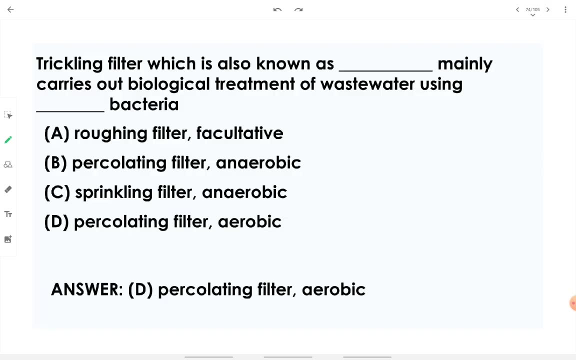 Okay, In trickling filter we carry out some kind of recirculation. Therefore, whatever the remaining biological content is there, it gets trapped over the stones. Okay, Fixed film growth carries out the biological treatment in trickling filter. Okay. 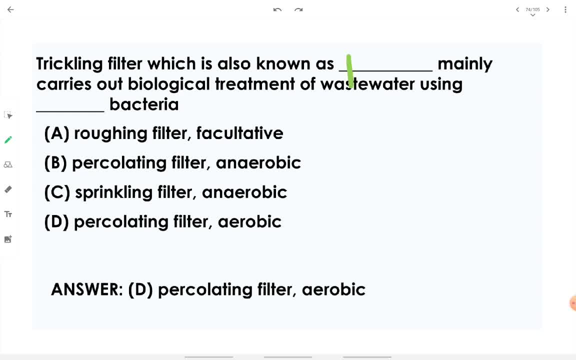 Trickling filter, which are also known as also called as percolating filter, mainly carry out biological treatment of wastewater using aerobic bacteria. Okay, Aerobic bacteria are the responsible one for carrying out biological treatment or oxidation of organic matter, which is given as input or feed water to trickling filter. 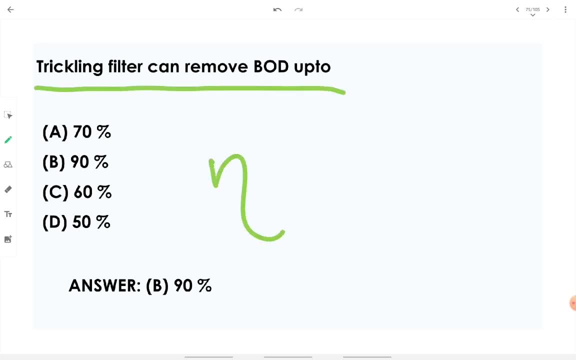 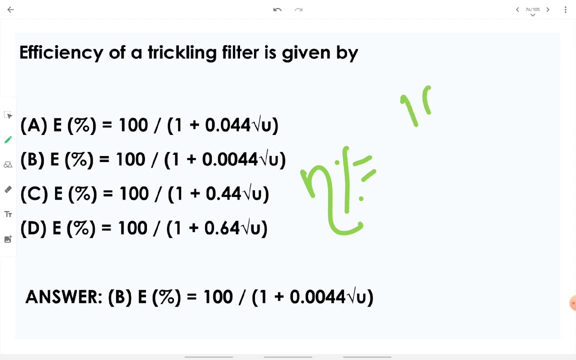 Then trickling filters: efficiency of BOD removal. its efficiency is 90 percent. Okay, TF removes 90 percent of BOD. Efficiency of trickling filter is given by: it is percentage efficiency and given by 100, divided by 1 plus 0.0044 square root of square root of U. 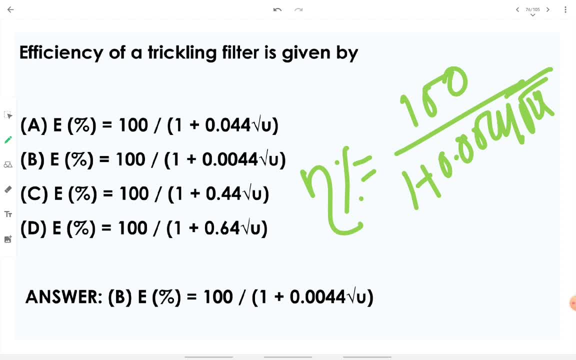 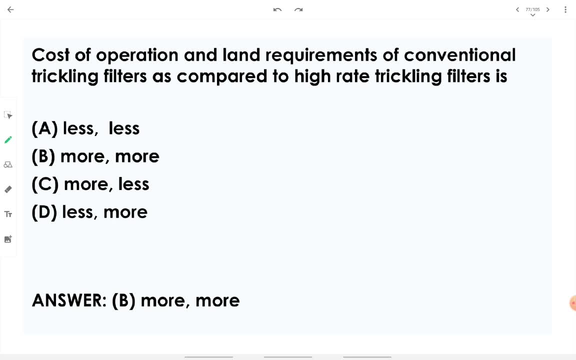 U is the rate of loading of wastewater inside the trickling filter, Then cost of operation and land requirement of conventional trickling filter is more and land requirement is also more. Both the thing means budget and space requirements of conventional trickling filter are more as compared to HRTF, which is high rate trickling filter. 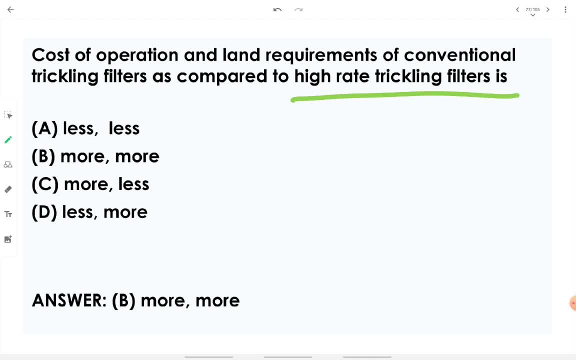 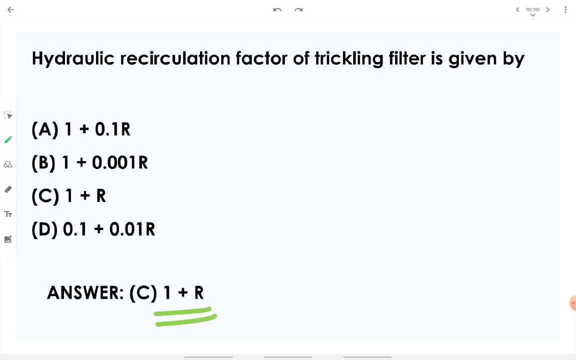 Therefore, when budget and space is a constraint is a worry, then we will always go with HRTF, that is, high rate trickling filter: Okay. Hydraulic recirculation factor of trickling filter is given by 1 plus R: Okay. 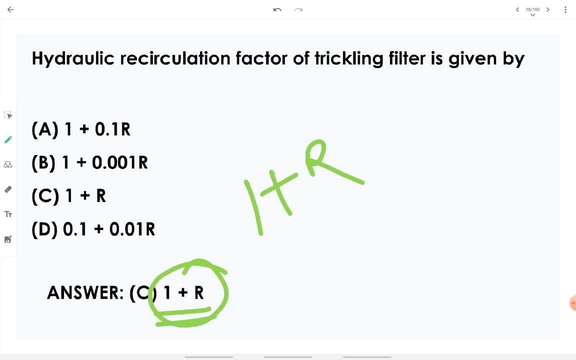 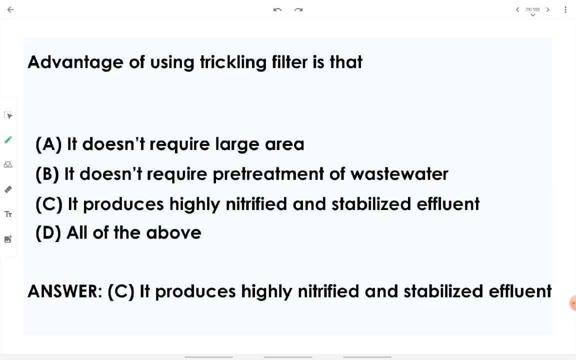 R is the rate of recycling or number we do. number of recycling is standing for R, Then advantage of using trickling filter is that it doesn't require large area. No, it does require large area. This is not the advantage. It doesn't require pretreatment. 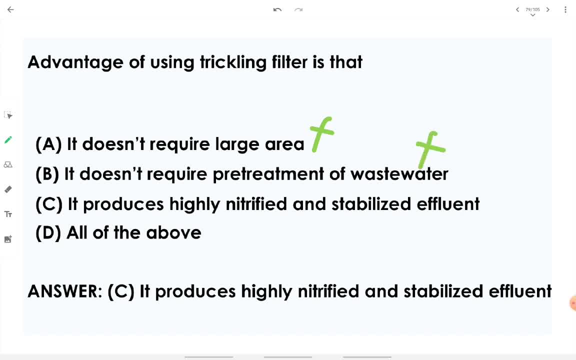 It does require pretreatment before you are letting wastewater to flow over trickling filter And you have to pretreat the wastewater. It produces highly nitrified and stable effluent. Yes, Stability of the effluent is very high when you are treating it with trickling filter. 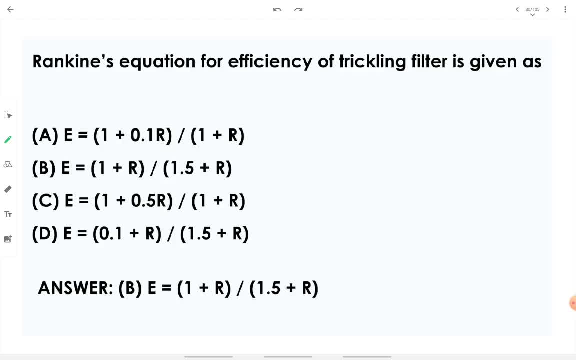 Okay, Therefore it is the advantage of trickling filter. Then Rankine's equation for efficiency of trickling filter is given as 1 plus R, divided by 1.5 plus R. This is the Rankine's equation of finding out efficiency of a trickling filter. 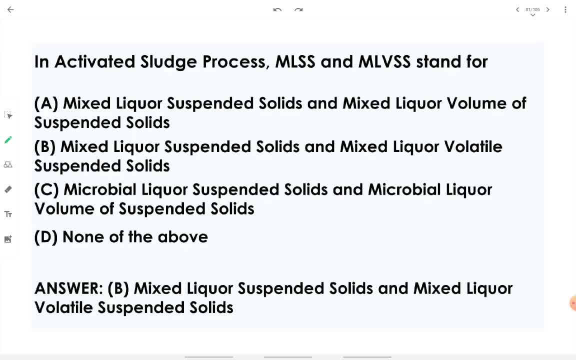 R means recirculation or recycling In activated sludge process. MLSS stands for Mixed Liquor Suspended Solid And MLVSS stands for Mixed Liquor Volatile Suspended Solid. Okay, Remember this: MLSS means Mixed Liquor Suspended Solid and MLVSS means Mixed Liquor Volatile Suspended Solid. 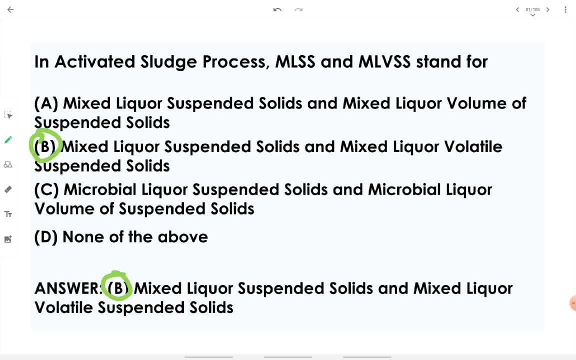 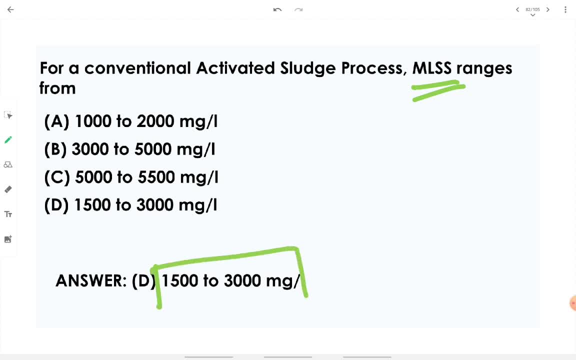 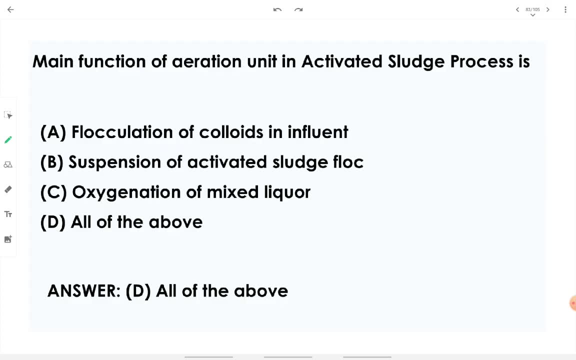 Option B is the correct answer here. For conventional activated sludge process, ASP, MLSS is 1500 to 3000.. Okay, Option D: 1500 to 3000 mg per liter or ppm. The main function of aeration unit in ASP is flocculation of colloid in influent. 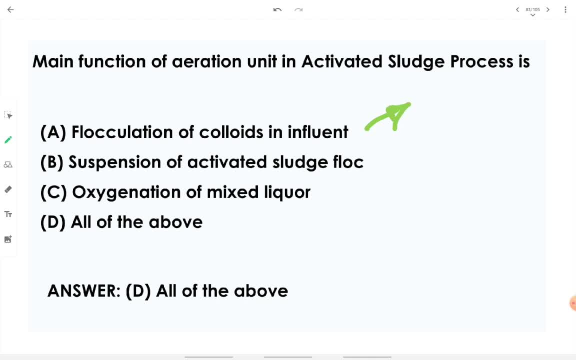 Yes, It causes flocc, formation of colloidal matter inside the influent. Then suspension of activated sludge: flocc, Okay, It causes, it keeps the activated sludge in suspended manner. Then, oxygenation of mixed liquor: Yes, The basic function is to provide oxygen. 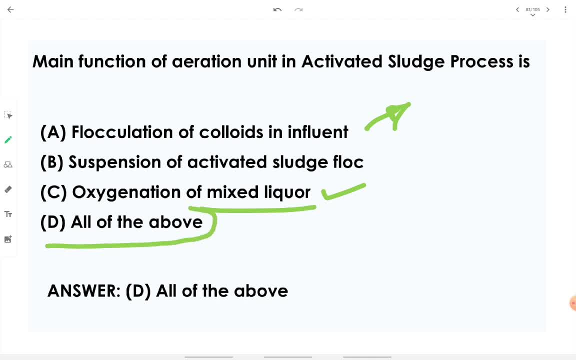 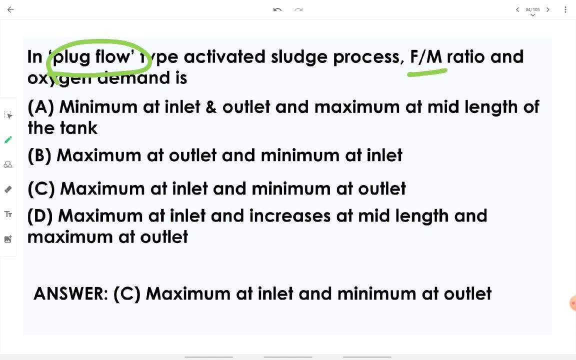 Therefore it causes oxygenation of mixed liquor. Therefore, all of the above mentioned factors are done by aeration unit in activated sludge process versus ASP. Option D should be the right answer. Then in plug flow type: activated sludge process. food to microorganism ratio. 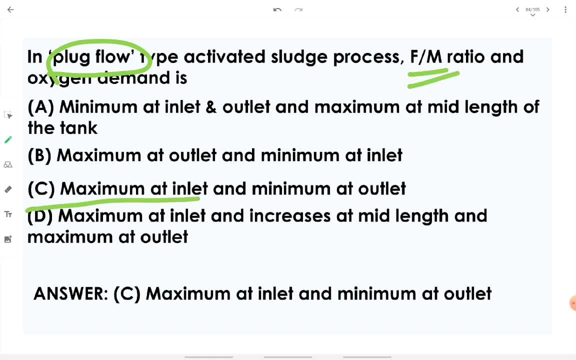 and oxygen demand is it is maximum at inlet And minimum at outlet. Okay, Plug flow means we are having a specific container in which wastewater is stored and then it is suddenly given to the unit. It is called a plug flow, And if we are having a pipeline that is continuously providing that, 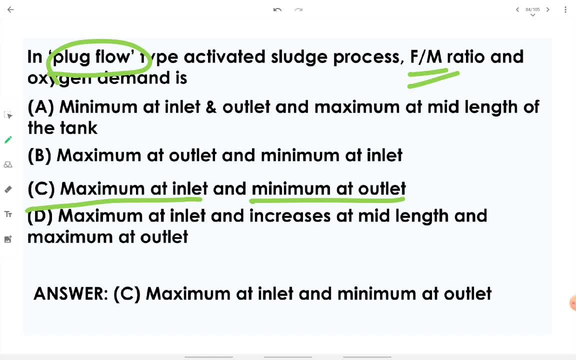 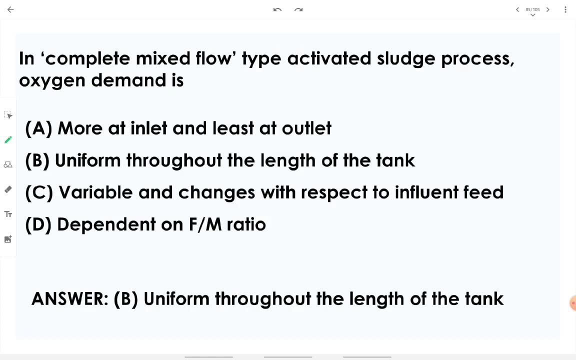 then it is continuous type of activated sludge process. Plug flow means store something in a container, then discharge it or let it in some treatment unit or any given unit. It is called a plug flow In complete mixed flow. type activated sludge process. oxygen demand is uniform throughout the length of the tank. 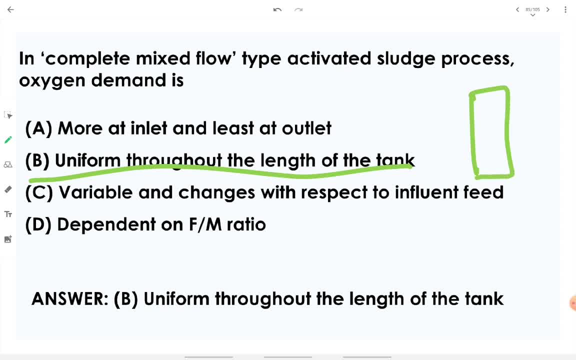 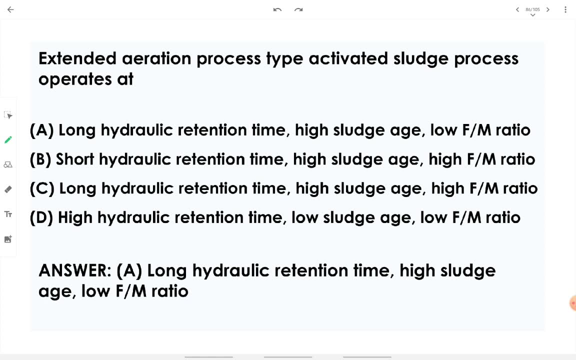 Okay Means, for example, this is the length of ASP, which is a complete mixed flow type. then aeration units have to be provided throughout the length of the ASP unit. Okay, Uniform throughout the length. Then extended aeration type: activated sludge process operates at long hydraulic. 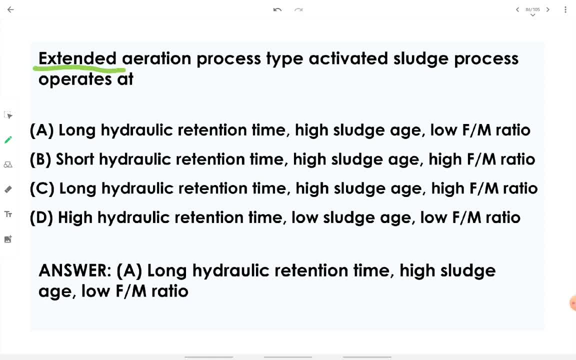 retention time. Obviously the world is suggesting more detention time, Okay, Or long hydraulic retention time. Then it has high sludge age. Age of the sludge in extended type is more. Then food to microorganism ratio required in extended ASP is low. 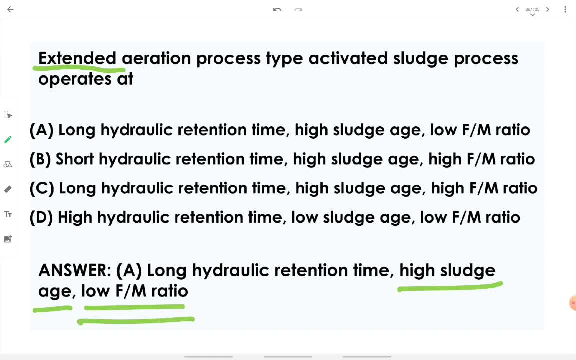 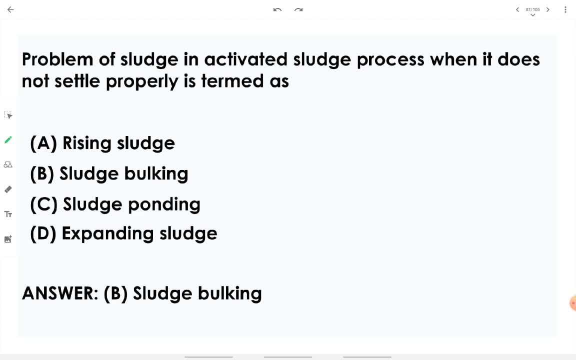 Okay, Low FM in extended aeration. Problem of sludge in activated sludge process, when it does not settle properly, is termed as sludge bulking. Okay, Sludge bulking is the trouble of ASP, In which it is not setting properly. 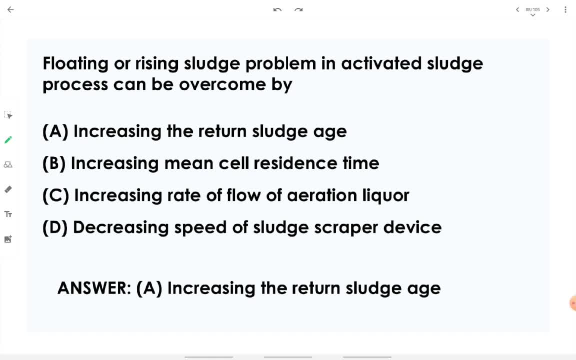 Then floating or rising sludge problem in activated sludge process can be overcome by increasing the return sludge age. whatever the recirculated sludge is, coming back to ASP, we have to provide more time it to set And then it can be introduced into the ASP zone. 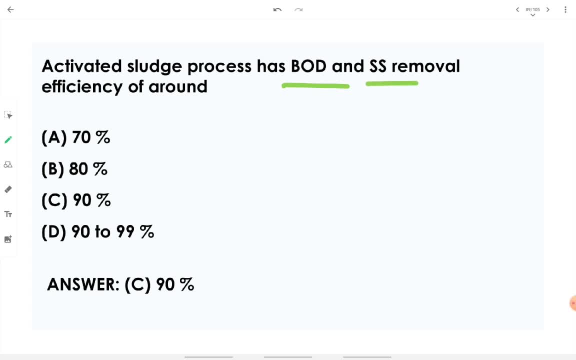 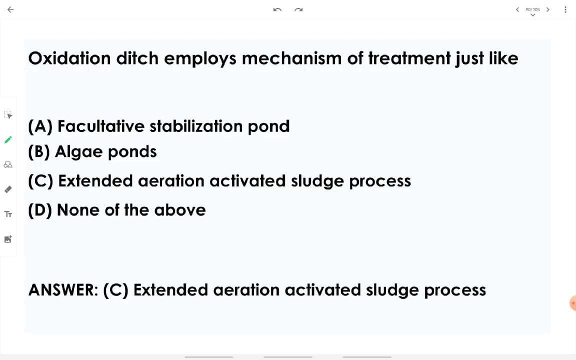 Activated sludge process has BOD and suspended removal efficiency of about 90%. Okay, ASP can remove 90% of BOD and suspended solids. Then oxidation ditch employs mechanism of treatment just like extended aeration activated sludge process- Okay, Oxidation ditch is nothing but recirculating. 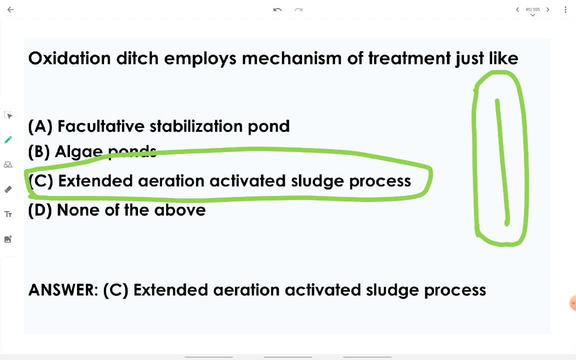 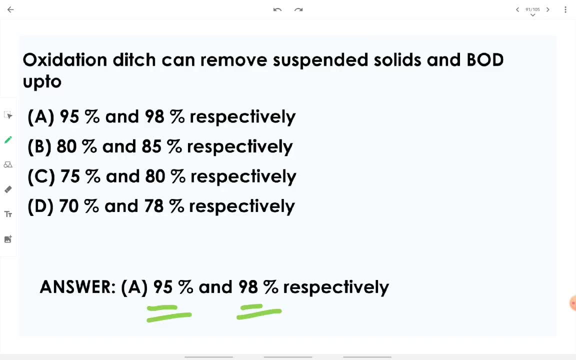 zone or oxidation ditch is there, in which what we are doing- We are providing aeration in it. Okay, It is employing the same mechanism as extended aeration ASP, in which we are having more hydraulic retention of wastewater. Oxidation ditch can remove suspended solids and BOD up to 95 to 98% respectively. 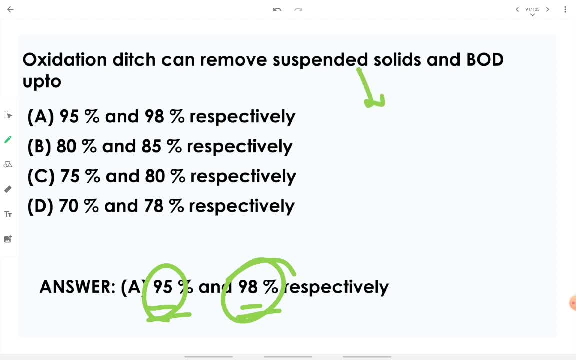 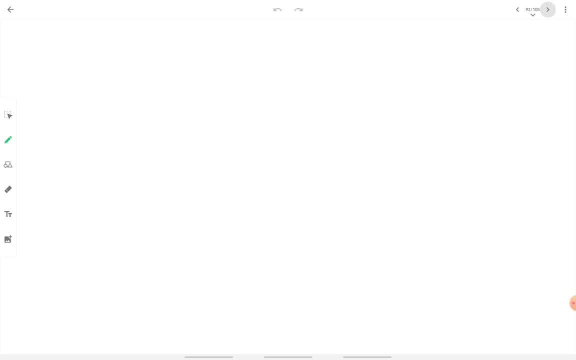 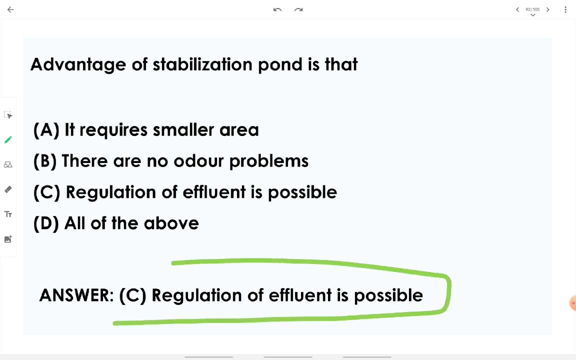 Okay, We can have SS to be removed up to 95% and BOD can be removed up to 98% in oxidation. ditch Stabilization pond has the advantage of regulating the effluent. Okay, Stabilization pond requires very vast area. 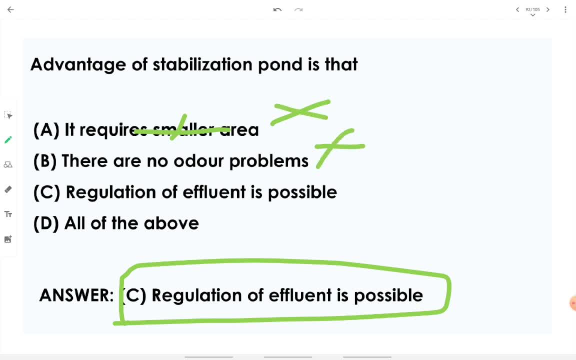 Therefore, this is not the answer. There are no odour problem. See, stabilization pond is open to atmosphere and whatever the digestion, whatever the process which are going over, the wastewater are exposed to the open atmosphere. Therefore there is odour problem and regulation of effluent. 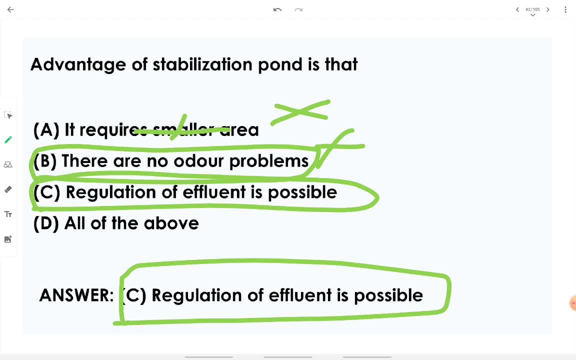 If possible, we can regulate. We can have more or less retention time: Okay. Hydraulic detention time in case of stabilization pond: Okay. Therefore, regulation of effluent with respect to quality and time of retention can be regulated. we can have a total control over it in stabilization pond. 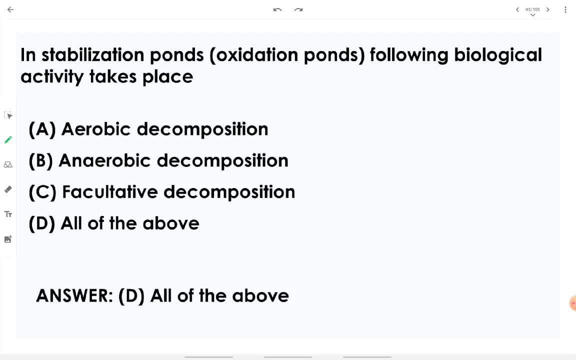 Then in stabilization, which is also known as oxidation pond. following is the biological activity that takes place inside it. Aerobic decomposition takes place in the upper layer of oxidation pond. Okay, Then anaerobic decomposition takes place at the bottom most layer and faculty. 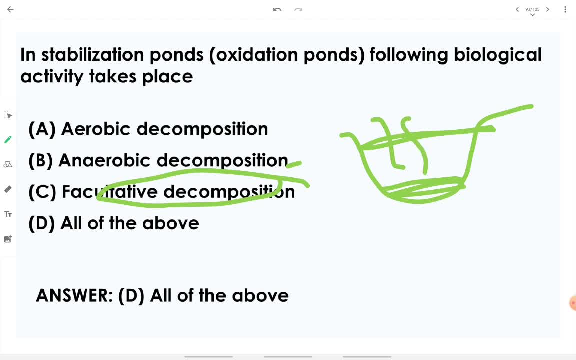 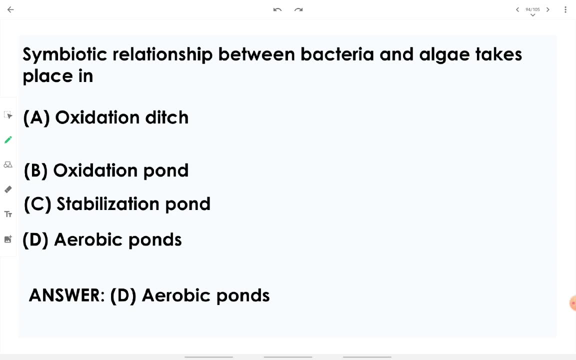 to decomposition takes place in the middle layer, where oxygen may or may not be present. Therefore all the kind of biological process- in absence, in presence or whatever with the situation of oxygen level- is there. it can be done in stabilization pond or oxidation pond. 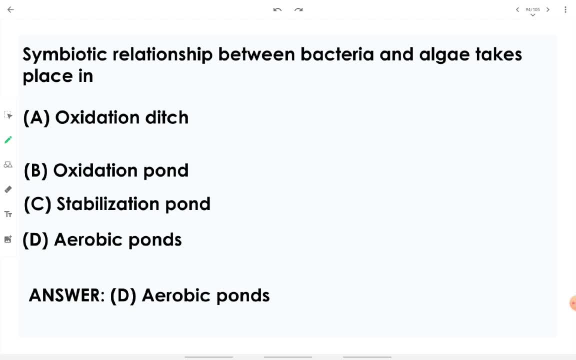 Symbiotic relationship. Okay, Symbiotic relationship means existence of some different kind of organism or living thing which are dependent on each other for their existence. Okay, It is the symbiotic relationship. Okay, They retrieve some benefits from each other and they coexist in the same environment. 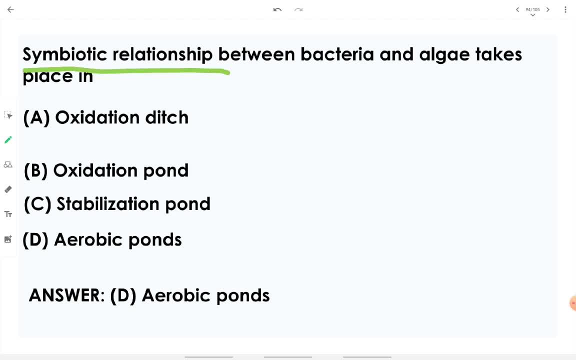 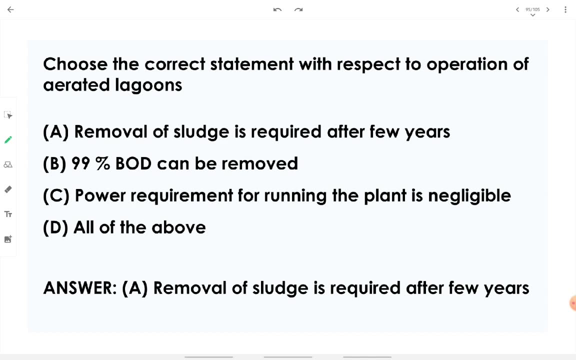 It is called a symbiotic relationship. Okay, Then it is between bacteria and algae that takes place. in which aerobic pond, In aerobic pond, symbiotic relationship between bacteria and algae exist. Choose the correct statement. with respect to operation of aerated lagoon. 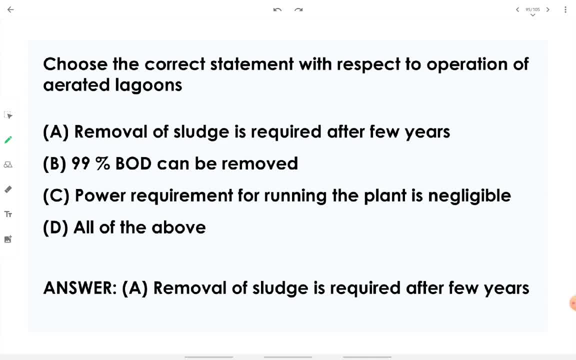 Okay, Removal of sludge is required after few years. Yes, you can rely on years long when it is about removal of sludge. 99% of BOD can be removed. No, it is not having that much efficiency. Then power requirement for running the plant is negligible. 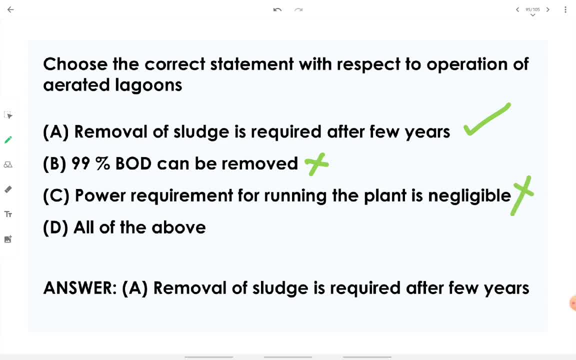 No, it is very wrong, because when we are talking about aerated lagoon, the vast tanks, the vast lagoons have to be provided with aeration techniques. Therefore it has more power requirement. Therefore, only option A is correct here. 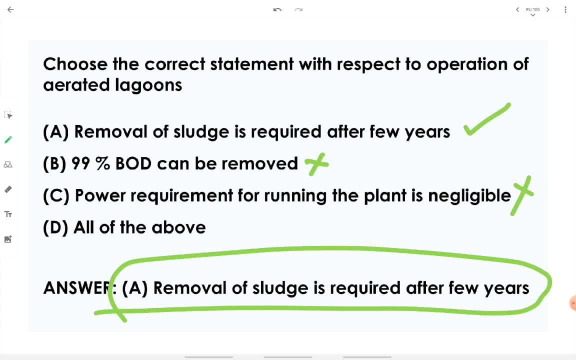 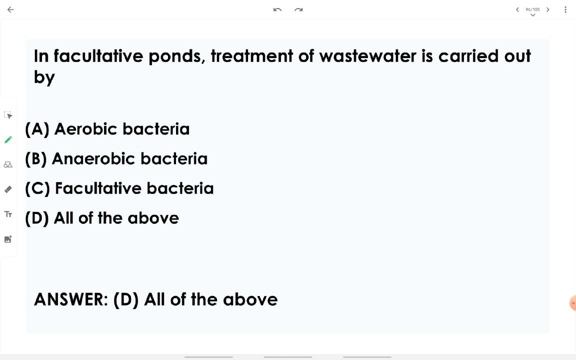 We can have the sludge removal process to take place after a period of years. Then in facultative pond, treatment of wastewater is carried out by gas In facultative pond. all the three processes in presence of oxygen, in absence of oxygen or whichever the condition prevails. 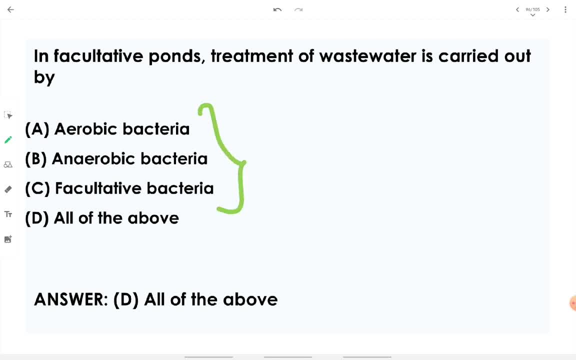 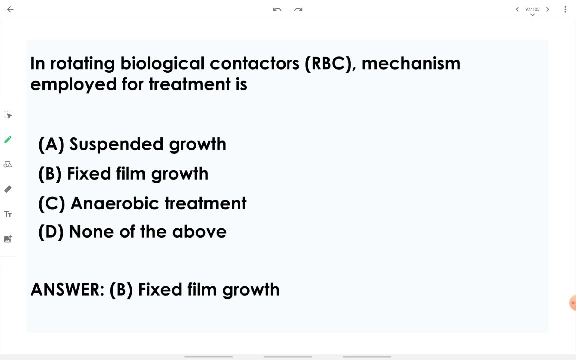 Which is facultative. Therefore, aerobic, anaerobic and facultative bacteria- all three kinds of bacteria can work in facultative pond for causing treatment of wastewater. All of the above is the right answer. here, In RBC, rotating biological contactor mechanism employed for treatment is: 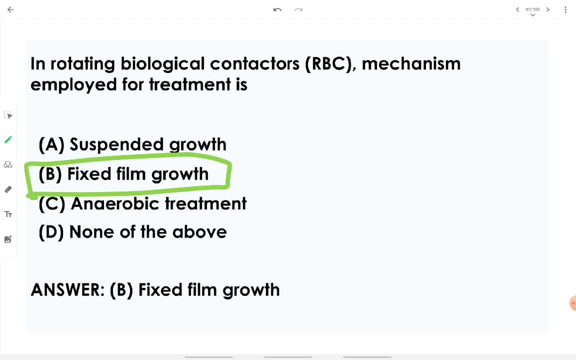 fixed film growth. Okay, what happens in RBC is, see, you have been provided with a container like this and then you have to treat the water by using RBC. What you are going to do, You are going to have a shaft over here, over the tank and over the shaft. 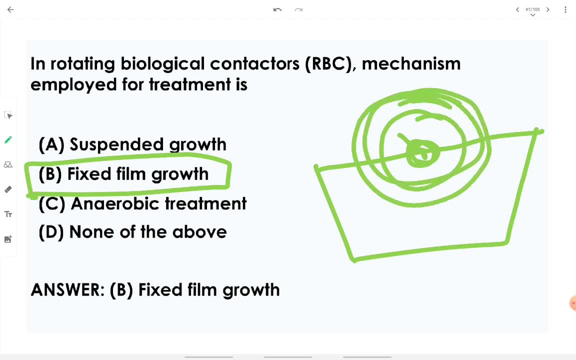 number of thin discs. number of thin discs are employed and a rotation with a small rpm, let's say three to five rpm, is given to the rotation of the disc. And what will happen? The disc will be having about 40 percent submergence in wastewater. 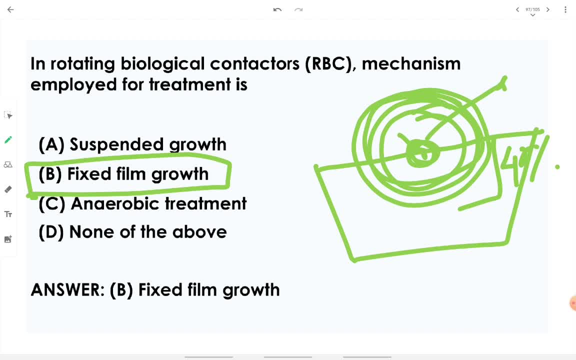 Now what will happen? The discs have their surface area very rough. Okay, now, over the rough surface area, the organic matter and bacteria which are present inside the wastewater will start culminating over there. Okay, they will start growing over the surface and then, whatever the media, 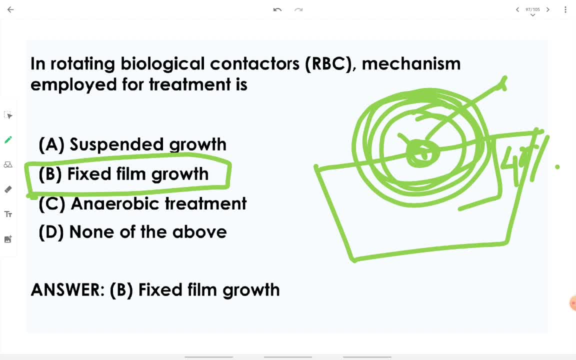 inside the disc or over the disc is there. the media will be accumulated with fixed film or biofilm over there. Now, because of the rotation, the disc will be exposed to atmosphere so that it can have O2 or oxygen or DO from the air and it will again go. 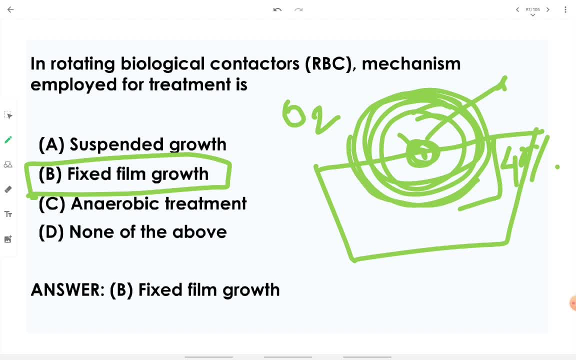 inside the wastewater to again get in contact with bacteria and organic matter. Therefore, this cycle goes on continuing And after a while the discs are very much populated with the bio or slimy film which is called the fixed film growth. Okay, there is no suspended growth promoted in RBC. 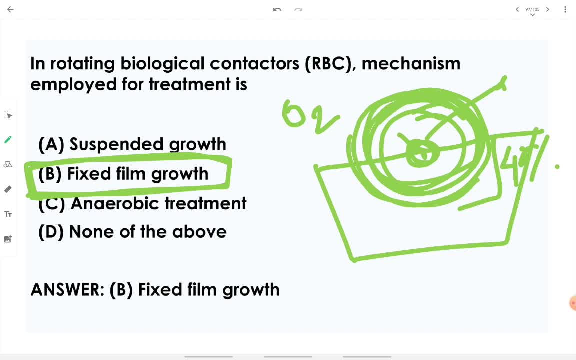 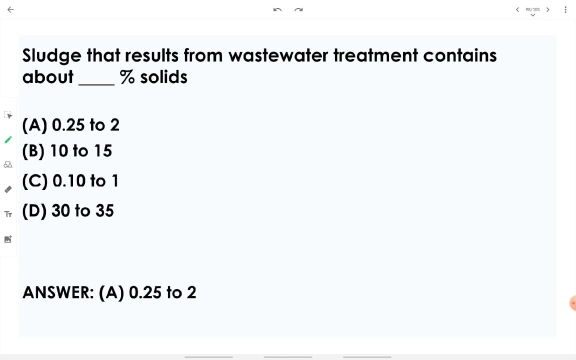 RBC and trickling filter have the fixed film growth mechanism. ASP, on the other hand, has suspended growth mechanism for biological action to take place. Okay, sludge that results from wastewater treatment contains about 0.25 to 2% solid. 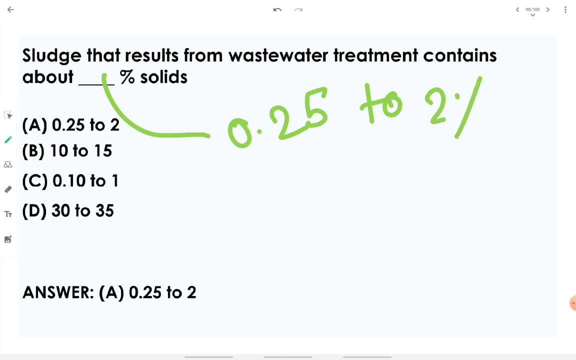 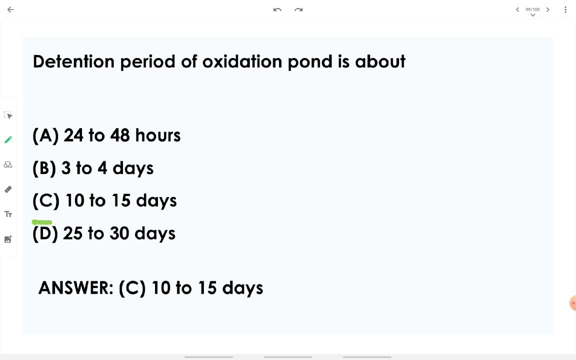 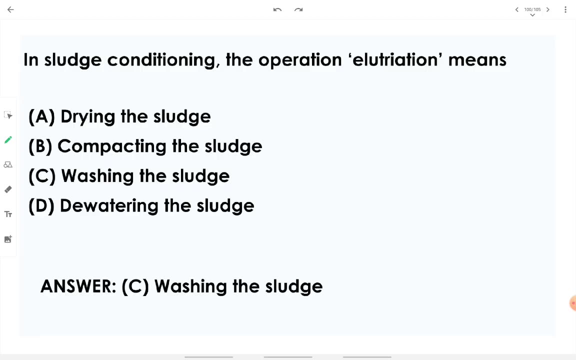 Okay, remember, 0.25 to 2% of solids. Okay then, detention period of oxidation pond is about 10 to 15 days. Oxidation pond DT is 10 to 15 days. Okay, in sludge conditioning the operation. alliteration means washing the sludge. 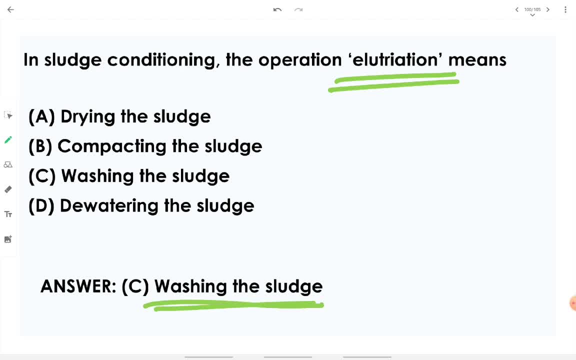 Okay, We wash the sludge so that we can get rid of some inorganic compounds from them. Okay, that's why we wash the sludge to get a cleaner, proper sludge over them. Okay, this is the sludge conditioning. 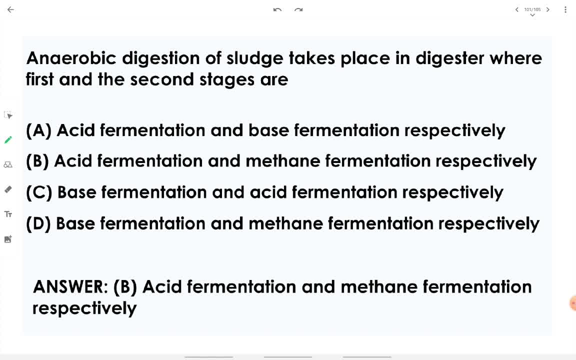 Okay, anaerobic digestion of sludge takes place in digester, where first and second stages are. The first stage will always be acid fermentation in the digester And the second stage will always be methane fermentation. Okay, AF and MF. AF and MF. 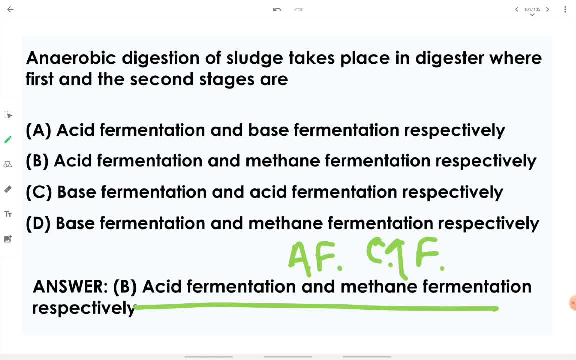 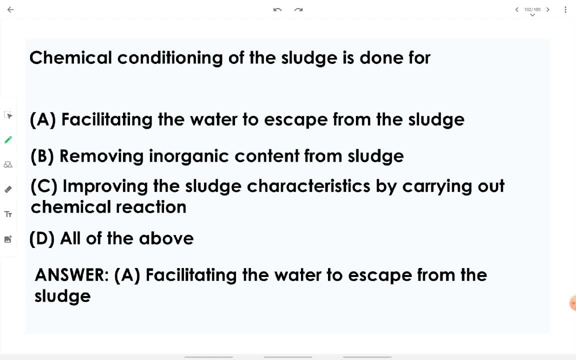 Remember, in anaerobic digestion of sludge, acid fermentation takes place first, methane fermentation takes place later. Okay, chemical conditioning of the sludge is done for facilitating the water to escape from the sludge. What we are doing in sludge conditioning. 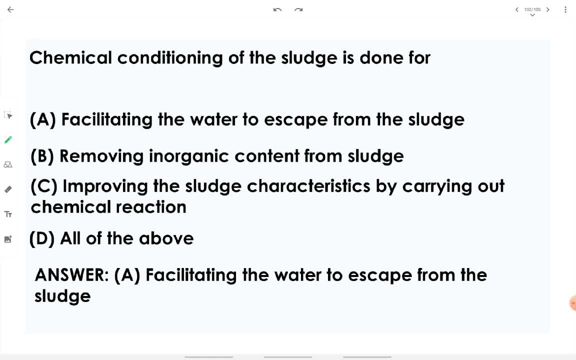 we are removing the sludge particle, that is, solid particle, from the wastewater and water is then separated. Okay, then adding the chemical causes the water particle to leave the sludge. Okay, therefore, solid sludge is separated and water is separated, And it can be done by adding some chemicals to the sludge. 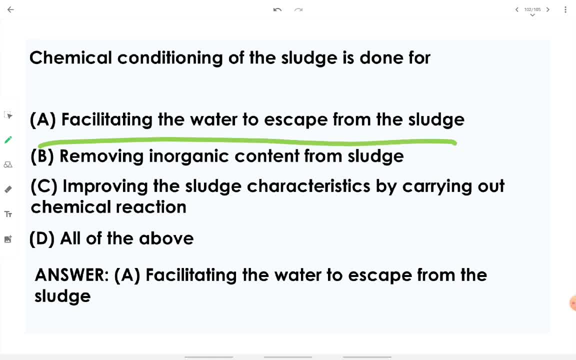 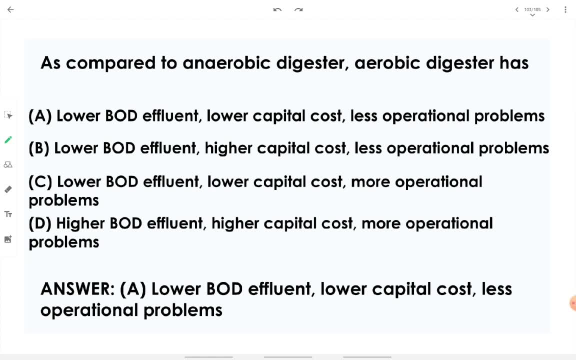 Okay, therefore, it is done for facilitating the water to escape from the sludge. As compared to anaerobic filter, aerobic digester has lower BOD effluent. Yes, anaerobic digestion has high BOD effluent, then less capital cost is. 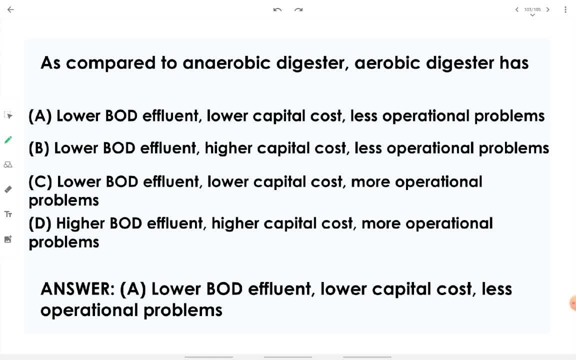 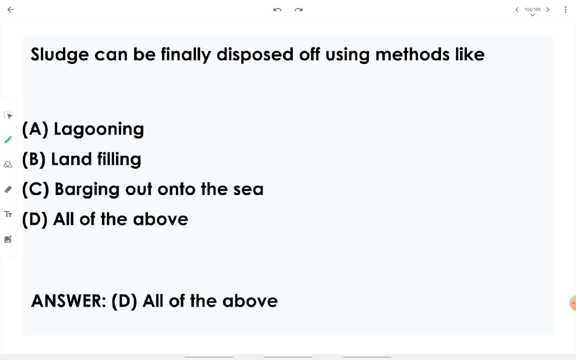 involved, Then less operational problems are there with respect to anaerobic digester in aerobic digester. Okay. therefore, option A is the correct one. Sludge can be finally disposed of by using method like: yes, you can go for aerated. 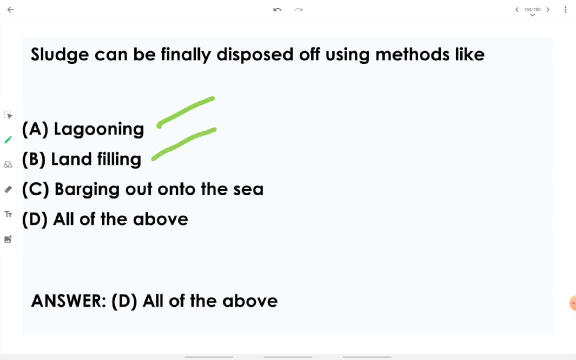 lagoons for sludge disposal, then you can have landfilling, sanitary landfill can be there. Then the third option is kind of conventional and old one which is not done nowadays but it was a method previously. It was a practice previously to let go the sludge off into the sea or ocean. 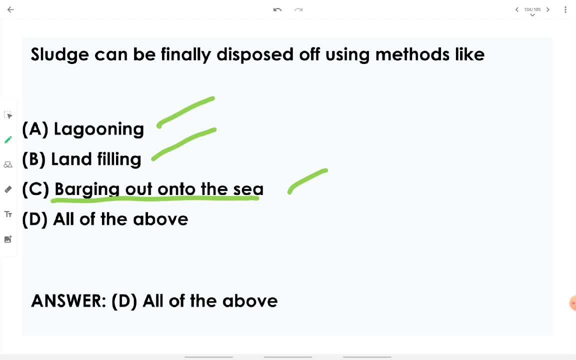 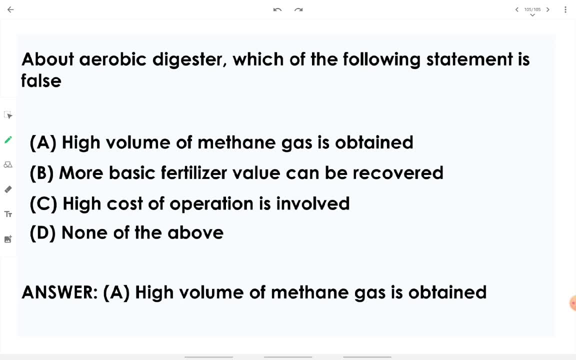 Okay, but still it is a process which was done. That's all of the work. should make the right answer here About aerobic digester. which of the following statement is false? Okay, in aerobic digester we do not get methane. 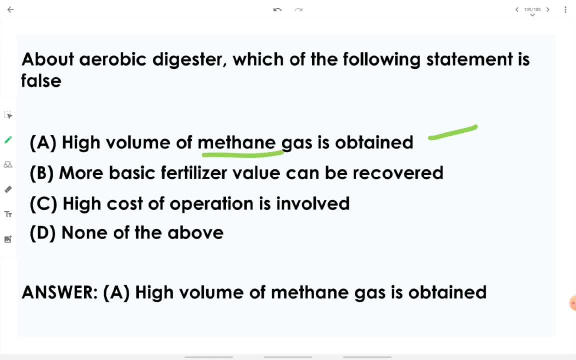 CH4 is not obtained in aerobic digestion. It is obtained in anaerobic digestion only. Therefore, this must be the answer. Check B and C and D. More basic fertilizer value can be recovered. Okay, High cost of operation is involved. 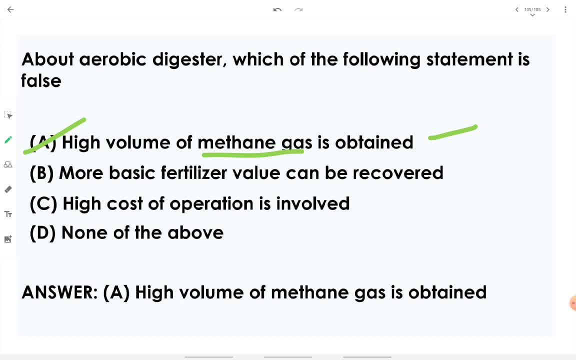 These are correct. regarding aerobic digester, The only incorrect statement is high volume of methane gas is obtained. Okay, option A make the right answer here. So that was the hundred plus questions series regarding wastewater engineering or sewage treatment. Okay, we will see. 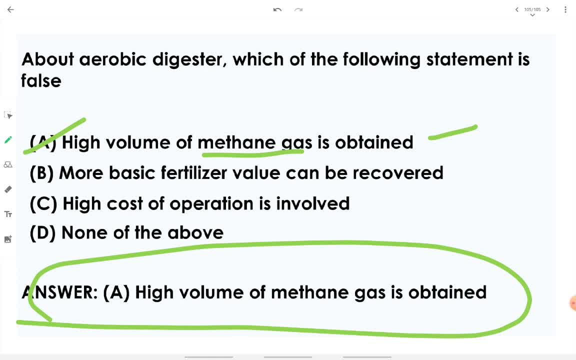 We will cover another topic in coming lecture. Till then, bye, Bye.